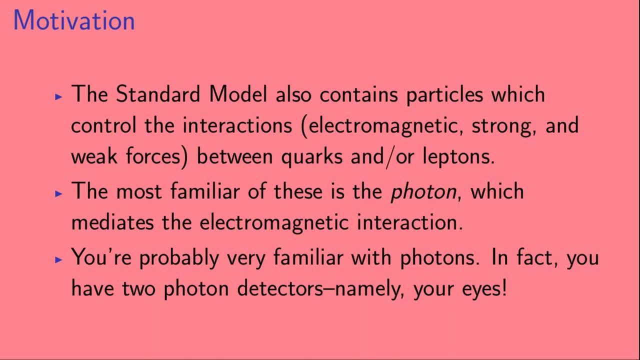 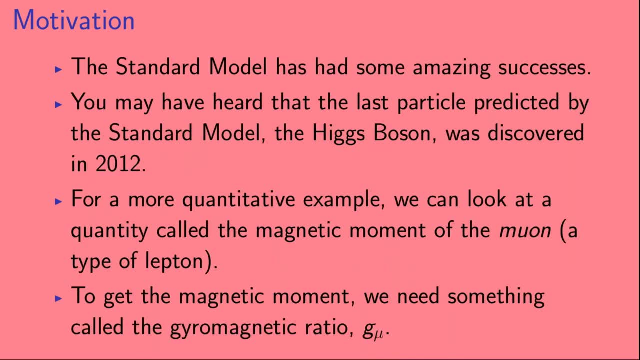 You're probably very familiar with photons. In fact, you have two photon detectors, namely your eyes. Now, the Standard Model has had some amazing successes. In fact, you have two photon detectors, namely your eyes. In fact, you have two photon detectors, namely your eyes. 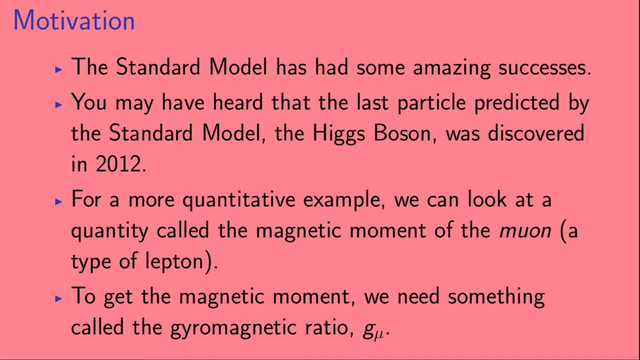 In fact, you have two photon detectors, namely your eyes. Six of these have extracted the force of the magnetic moment. You may have heard that the last particle predicted by the Standard Model, the Higgs boson, was discovered in 2012.. 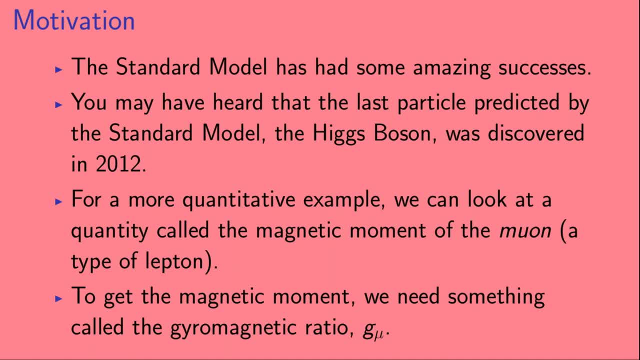 For a more quantitative example, we can look at a quantity called the magnetic moment of the muon, and the muon is a type of lepton. To get the magnetic moment we need something called the gyromagnetic ratio, g sub mu. 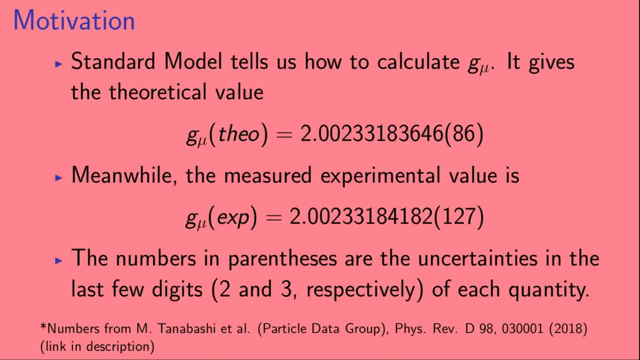 The standard model tells us how to calculate g sub mu. It gives the theoretical value shown here 2.00233183646.. Meanwhile, the measured experimental value is something very similar. Here I should mention that the numbers in parentheses are the uncertainties in the last few digits. 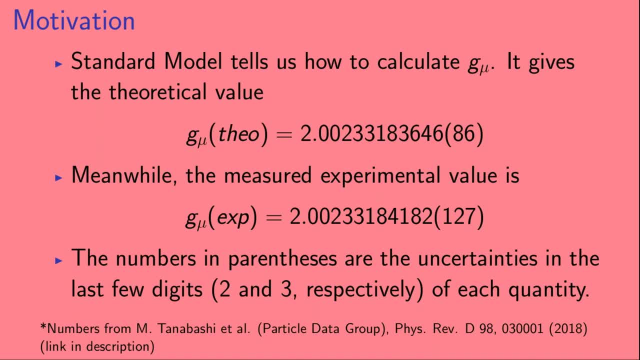 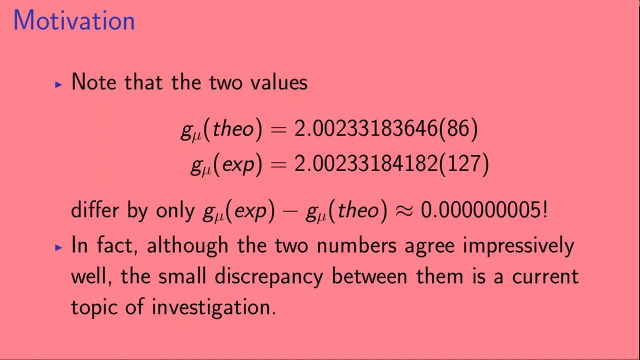 The last two digits or the last three digits, respectively, of each of these quantities. Now let's note that the two values, the theoretical value and the experimental value, differ by only 5 times 10 to the minus 9.. Actually, in fact, although the two numbers agree impressively well, 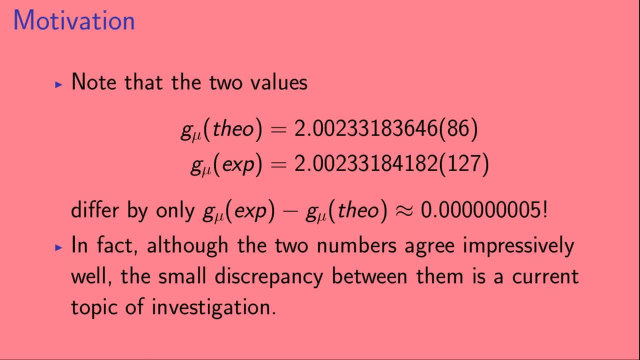 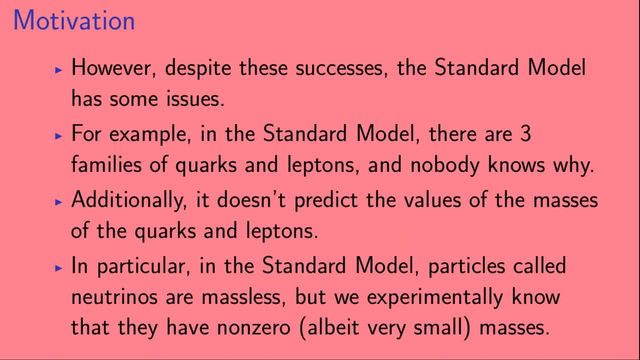 the small discrepancy between them is a coincidence. This is the current topic of investigation. Despite these successes, the standard model has some issues. For example, in the standard model there are three families of quarks and leptons and nobody knows why. 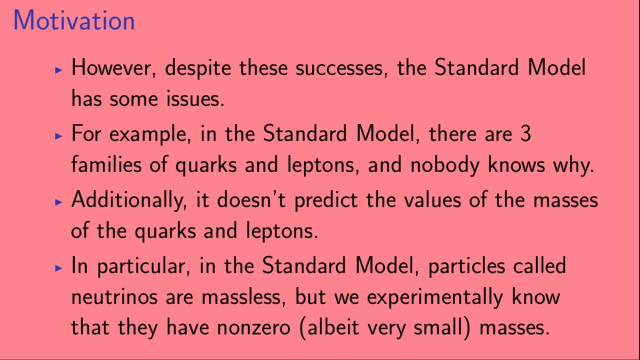 Additionally, it doesn't predict the values of the masses of the quarks and leptons In particular. in the standard model, particles called neutrinos are massless, but we expect them to be massless. We experimentally know that they have non-zero, although very small, masses. 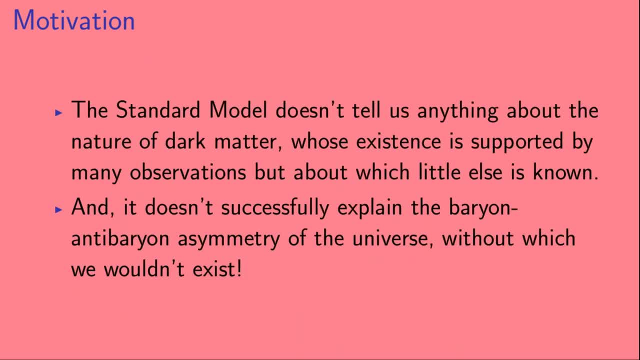 The standard model also doesn't tell us anything about the nature of dark matter, whose existence is supported by many observations but about which little else is known, And it doesn't successfully explain the baryon-antibaryon asymmetry of the universe. 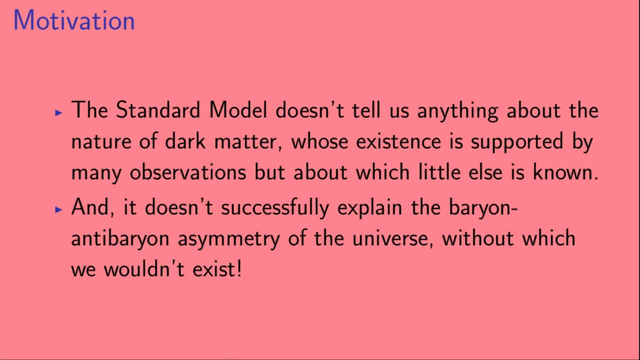 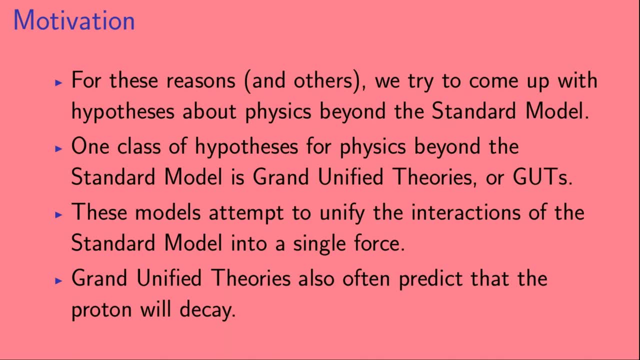 without which we wouldn't exist. For these reasons, among others, we try to come up with hypotheses about physics beyond the standard model. One class of hypotheses for physics beyond the standard model is grand unified theories, or GUTS. These models attempt to unify the interactions of the standard model into a single force. 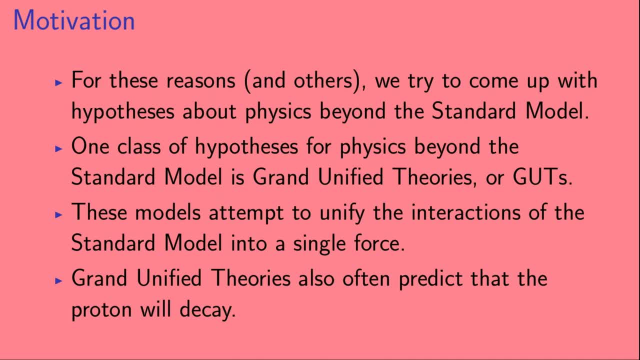 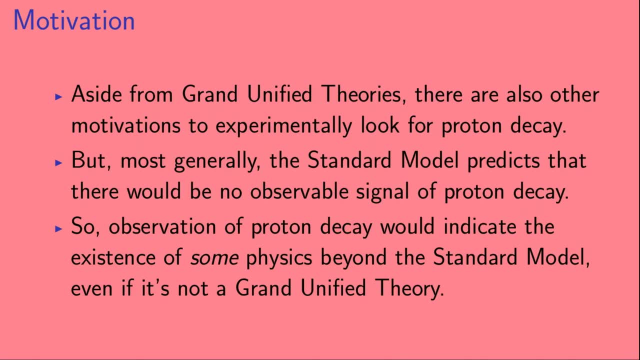 Grand unified theories also often predict that the proton will decay. Aside from grand unified theories, there are also other motivations to experimentally look for proton decay. But most generally the standard model predicts that there would be no observable signal of proton decay. 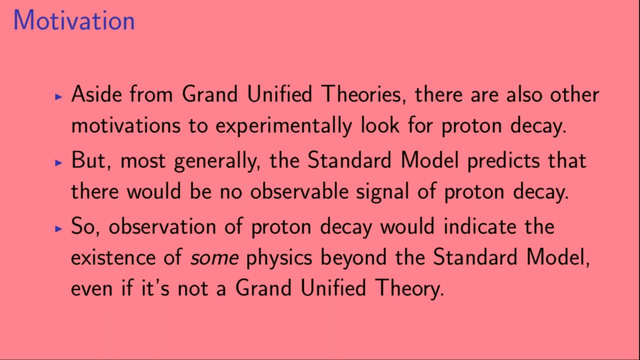 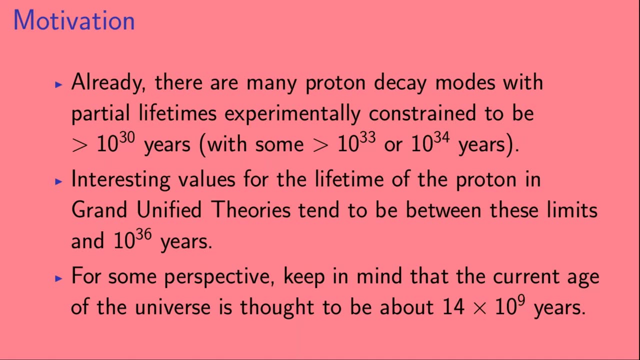 So observation of proton decay would indicate the existence of some physics beyond the standard model, even if it's not a grand unified theory. Already there are many proton decay modes with partial lifetimes experimentally constrained to be greater than 10 to the 30 years. 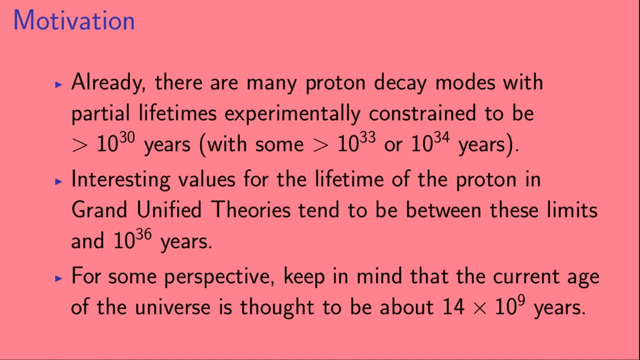 And some of those are constrained to be greater than 10 to the 33 or 10 to the 34 years. Interesting values for the lifetime of the proton in grand unified theories tend to be between these limits and 10 to the 36 years. 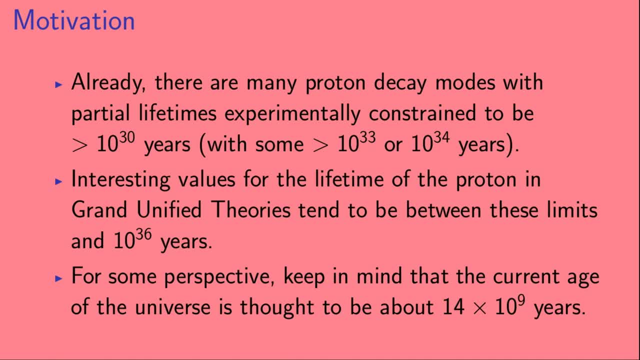 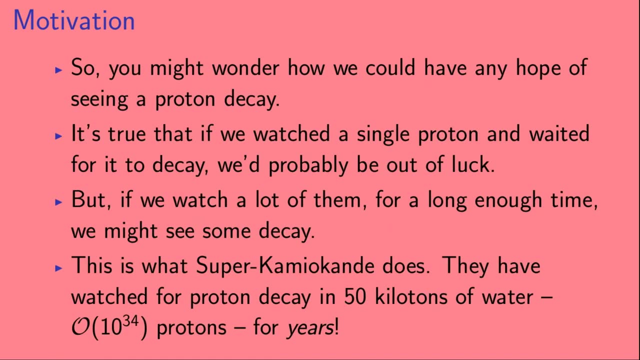 For some perspective. keep in mind that the current age of the universe is thought to be only about 14 times 10 to the 9 years. So you might wonder how we could have any hope of seeing a proton decay. It's true that if we watched a single proton and waited for it to decay, 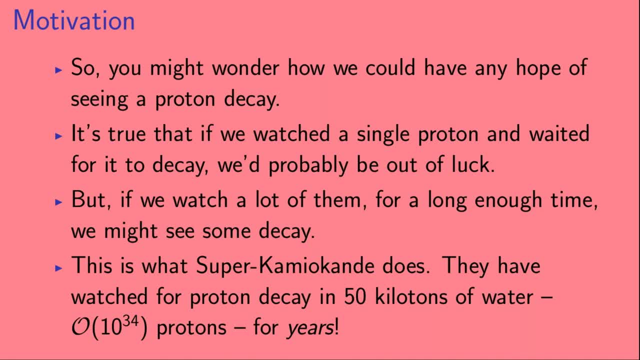 we'd probably be out of luck. But if we watch a lot of protons and a lot of them for a long enough time, we might see some decay. This is what Super-Kamiokande does. They have watched for proton decay in 50 kilotons of water. 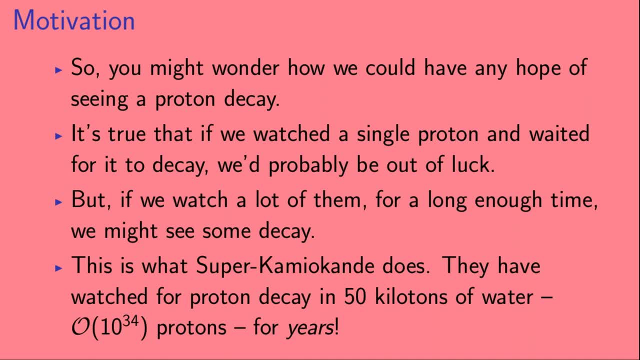 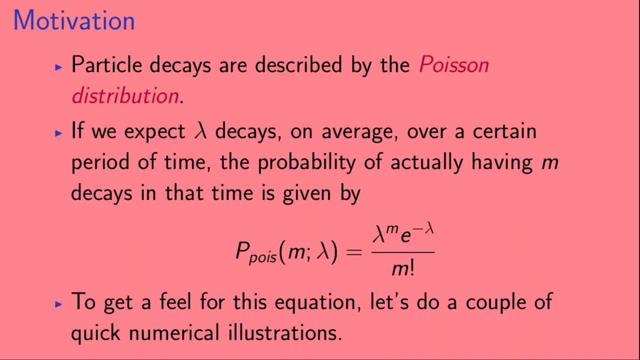 which is of order 10 to the 34 protons, and they've been watching them for years Now. particle decays are described by the Poisson distribution. If we expect lambda decays on average over a certain period of time, the probability of actually having m decays in that time. 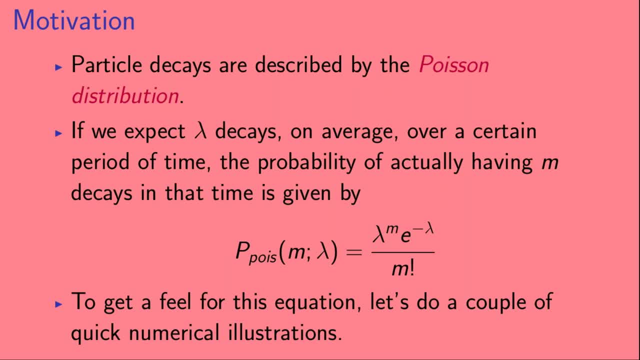 is given by the Poisson distribution. So P Poisson of m given lambda, which is equal to lambda, to the m e to the minus lambda divided by m factorial. To get a feel for this equation, let's do a couple of quick numerical illustrations. 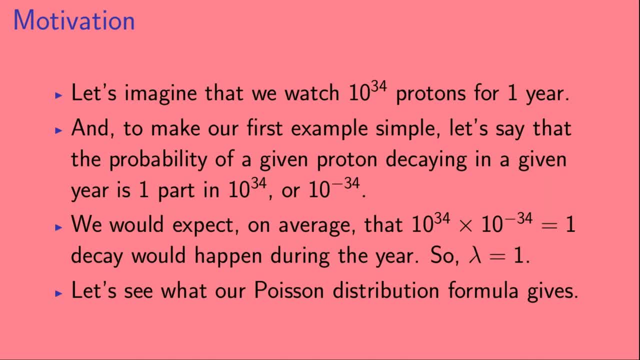 So let's imagine that we watch 10 to the 34th protons for one year And to make our first example simple, let's say that the probability of a given proton decaying in a given year is one part in 10 to the 34,. 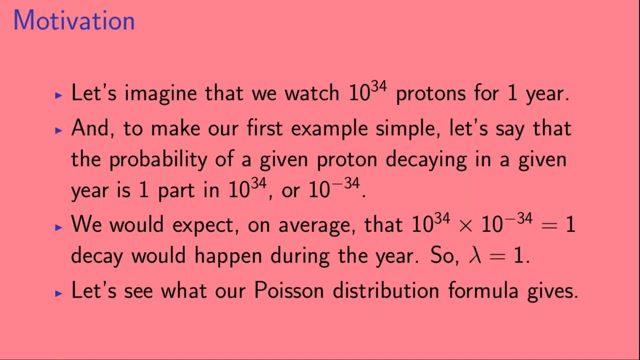 or 10 to the minus 34.. We would expect on average that 10 to the 34 times 10 to the minus 34,- that's equal to one decay- would happen during the year. So lambda equals one. 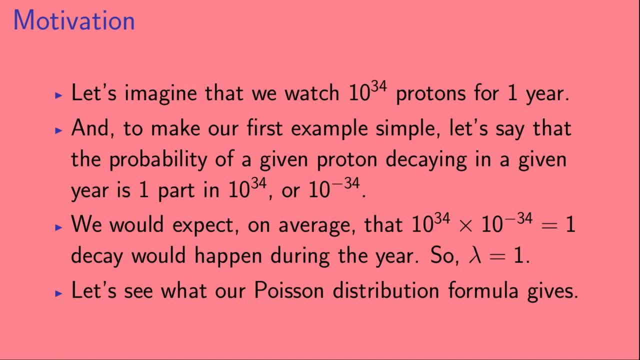 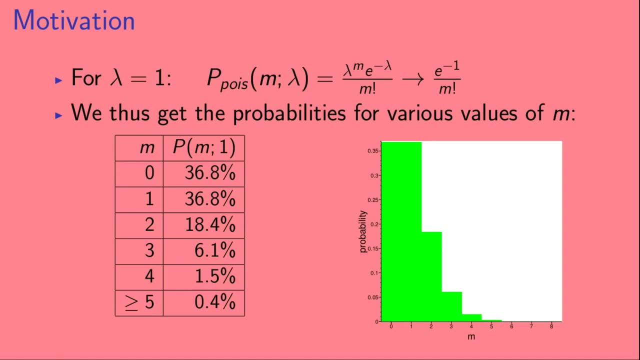 Let's see what our Poisson distribution formula gives. Okay, so for lambda equal to one, our Poisson formula- lambda to the m, e to the minus lambda over m factorial- just becomes e to the minus one over m factorial. 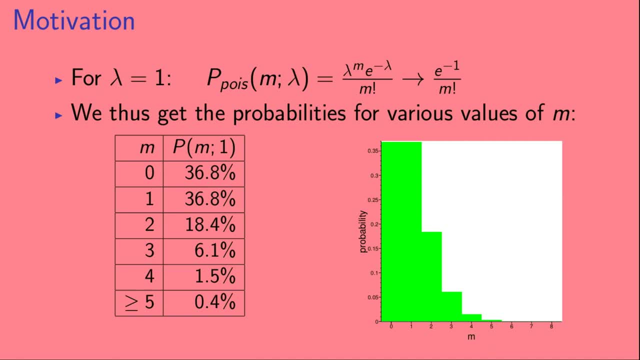 We thus get the following probabilities for various values of m. So the probability of m being zero- so that's seeing zero events- is 36.8%. The probability of seeing one event is also 36.8%. The probability for seeing two events. 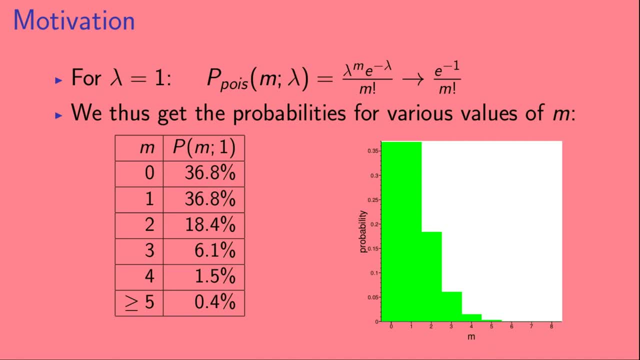 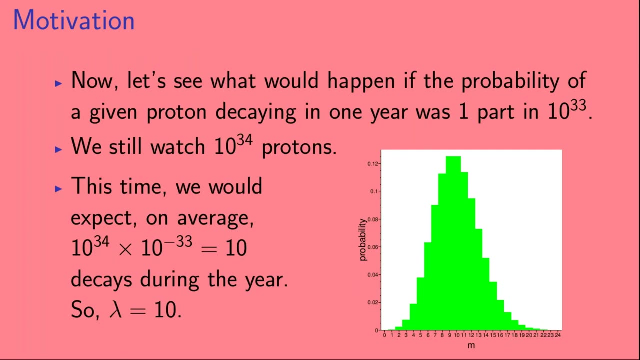 that's m, equals two is 18.4%, and so on. These values are illustrated in the plot at right. Now let's see what would happen if the probability of a given proton decaying in one year was one part in 10 to the 33.. 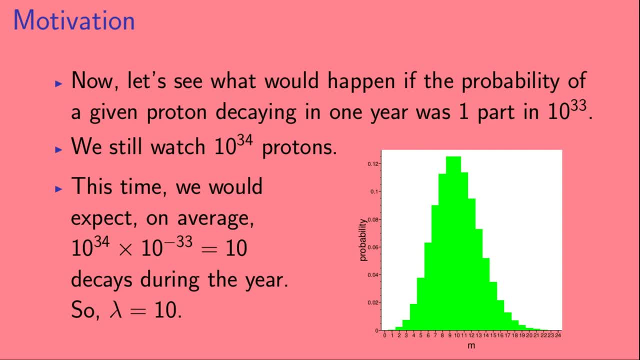 So we still watch. 10 to the 34 protons. 10 to the 34 protons. This time. we would expect, on average, 10 to the 34 times 10 to the minus 33,, which equals 10,. 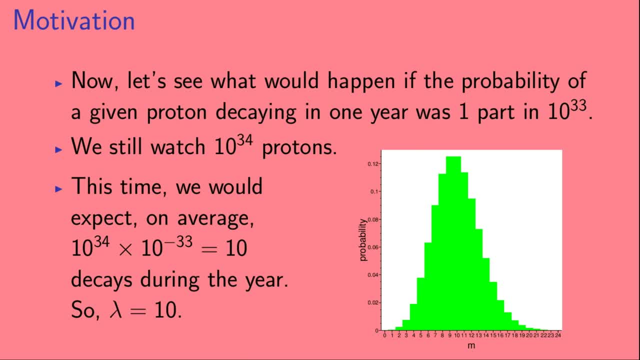 decays during the year. So lambda equals 10.. In the plot at right we show the probability to obtain m decays during the year. We see that it peaks around m equals 10, but the values of m greater than 10. 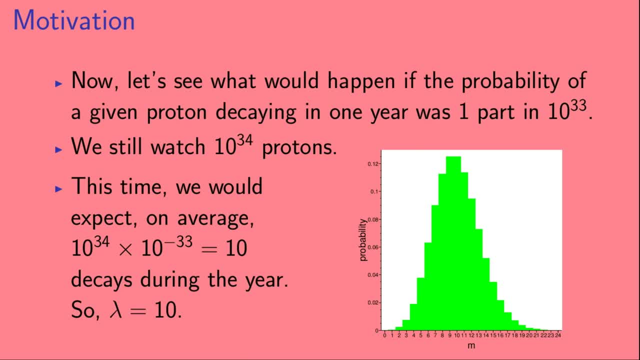 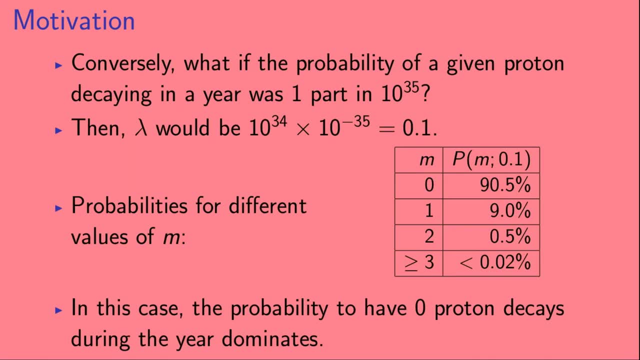 and less than 10 are both still allowed, Okay. Conversely, what if the probability of a given proton decaying in a year was one part in 10 to the 35? Then lambda would be 10 to the 34 times 10 to the minus 35,. 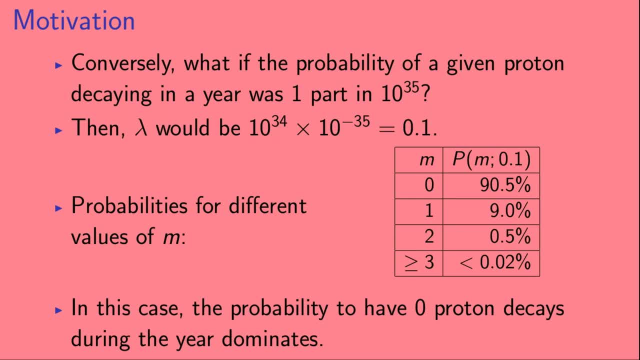 which equals 0.1.. So here we give a table of probabilities for different values of m. We can see that the probability to have m equals 0, that's to see 0 decays is 90.5%. The probability to see 1 decay 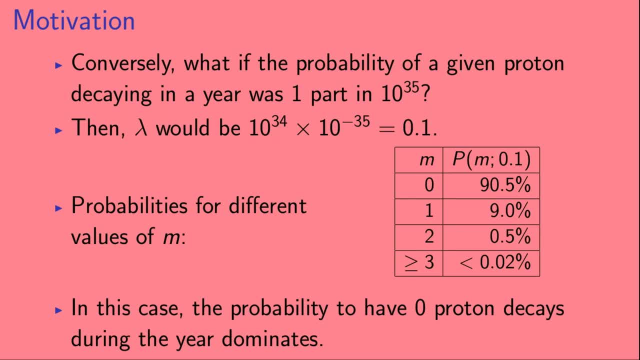 is 9%. The probability to see 2 decays is 0.5% and the probability to see more than 2 decays is quite small. In this case, the probability to have 0 proton decays during the year dominates. 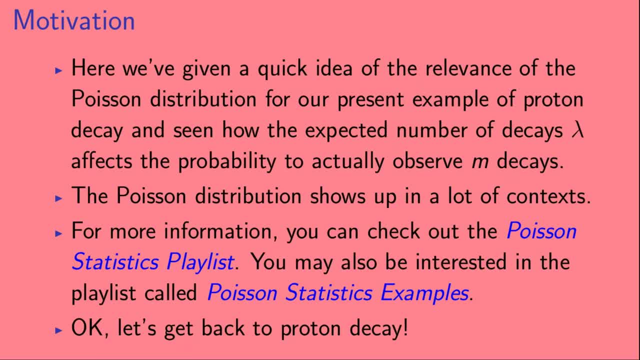 Okay. So here we've given a quick idea of the relevance of the Poisson distribution for our present example of proton decay, and we've seen how the expected number of decays lambda affects the probability to actually observe m decays. Now the Poisson distribution shows up. 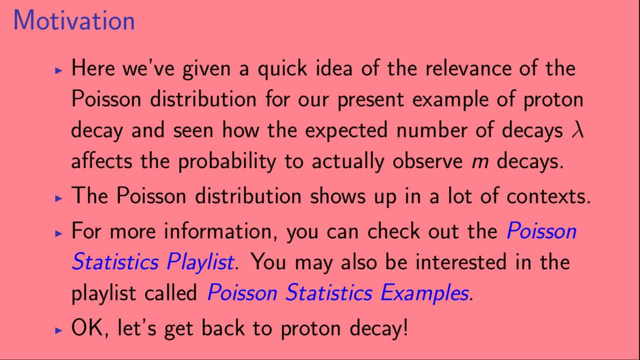 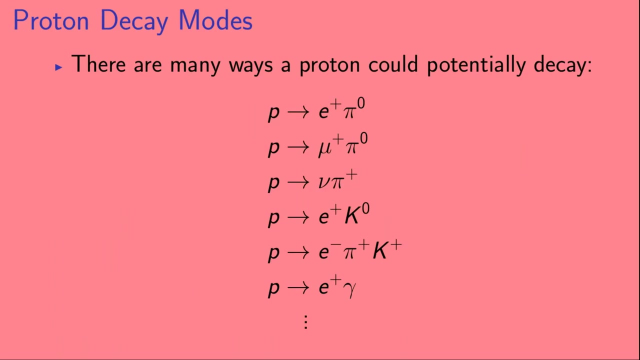 in a lot of contexts. For more information, you can check out the Poisson statistics playlist. You may also be interested in the playlist called Poisson statistics examples. Okay, Let's get back to proton decay. So there are many ways a proton could potentially decay. 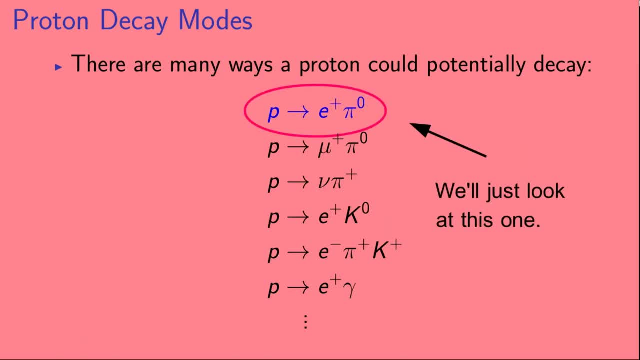 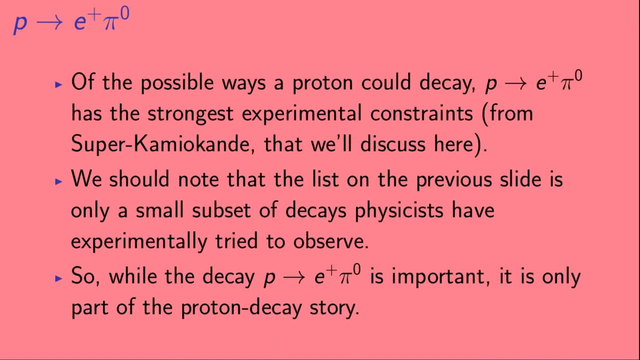 Here we'll just look at this first one. P goes to E plus pi-naught. Here the E plus is a particle known as the positron, and the pi-naught is a neutral meson Of the possible ways a proton could decay. 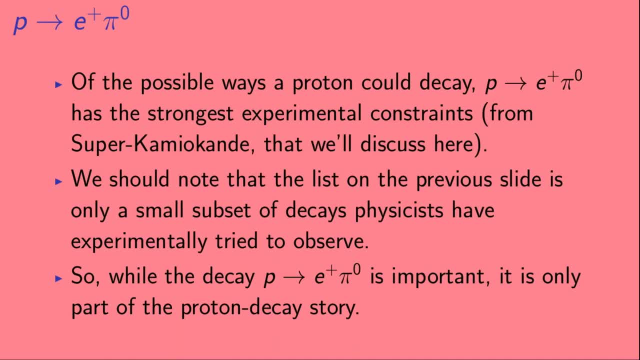 P goes to E plus pi-naught has the strongest experimental constraints. In fact, those are the experimental constraints from Super-Kamiokande that we'll discuss here. We should note that the list on the previous slide is only a small subset of decays. 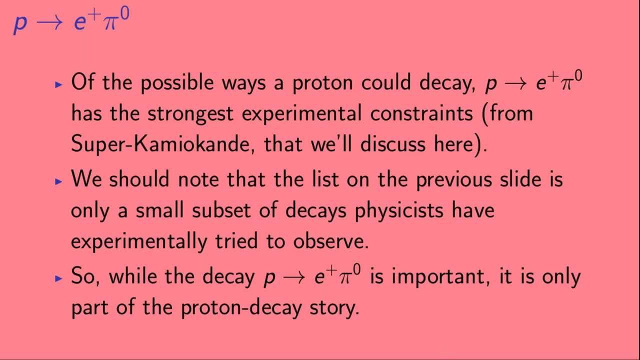 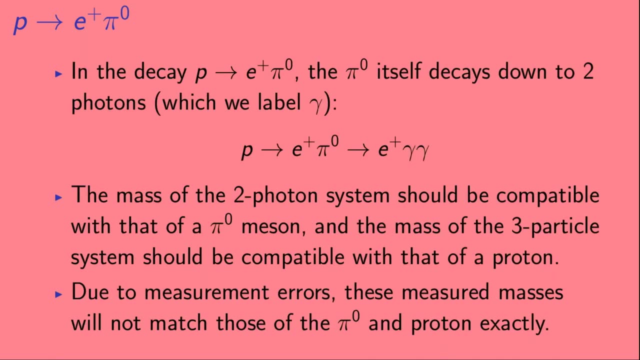 physicists have experimentally tried to observe. So while the decay P goes to E plus pi-naught is important, it is only part of the proton decay story. In the decay P goes to E plus pi-naught, the pi-naught itself decays down to two photons. 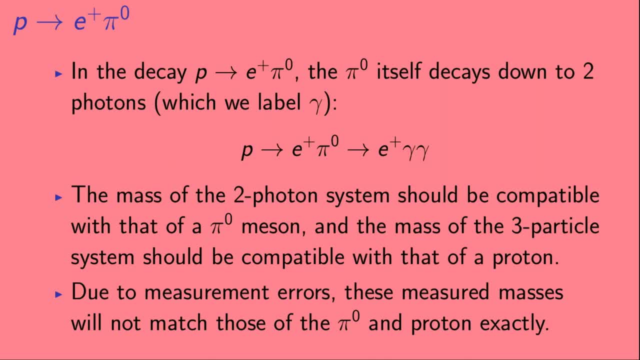 which we label as gamma. So we end up with: P goes to E plus pi-naught, which goes to E plus gamma-gamma. The mass of the two-photon system should be compatible with that of a pi-naught meson. 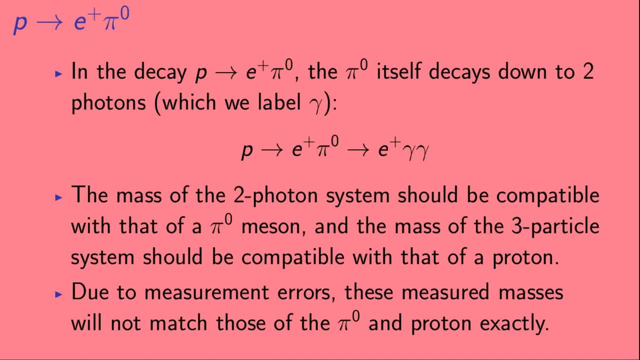 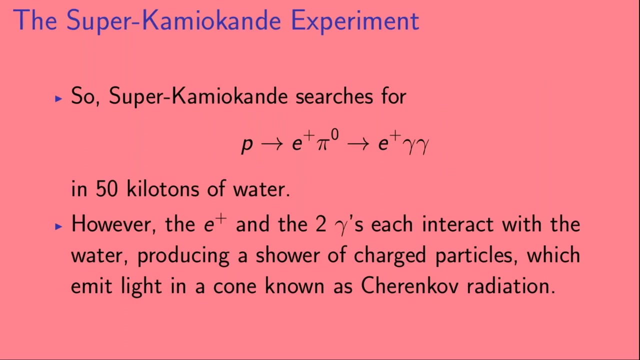 and the mass of the three-particle system should be compatible with that of a proton. Due to measurement errors, these measured masses will not match up those of the pi-naught and proton. exactly Okay, so Super-Kamiokande searches for P goes to E plus pi-naught. 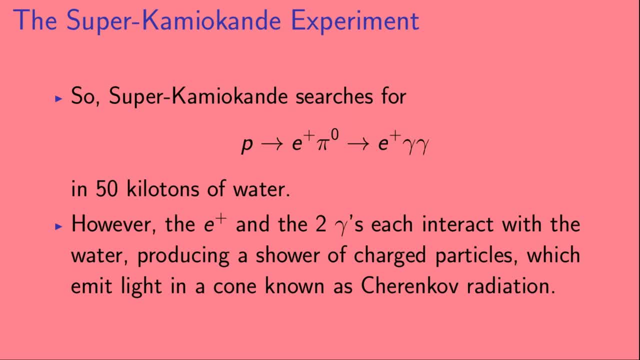 which goes to E plus gamma-gamma in 50 kilotons of water. However, the E plus and the two photons each interact with the water, producing a shower of charged particles which emit light in a cone known as Cherenkov radiation. 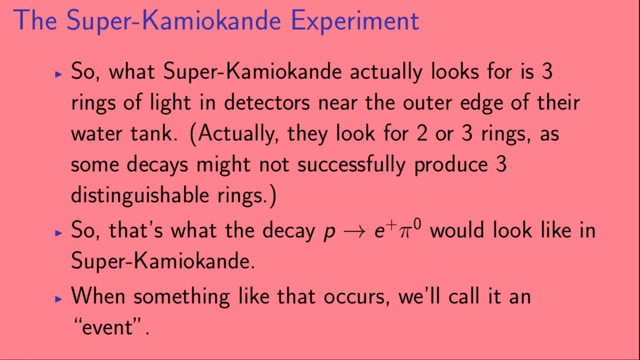 So what Super-Kamiokande actually looks for is three rings of light in detectors near the outer edge of their water tank, And actually they look for two or three rings, as some decays might not successfully produce three distinguishable rings. 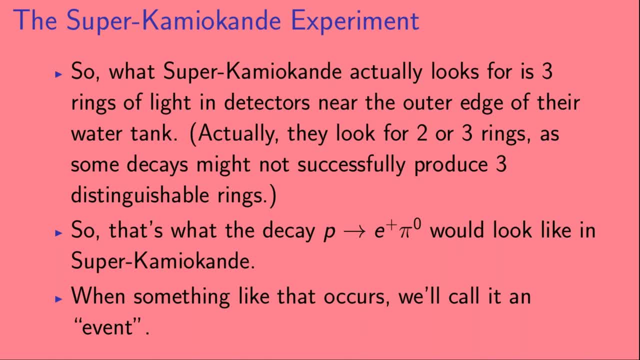 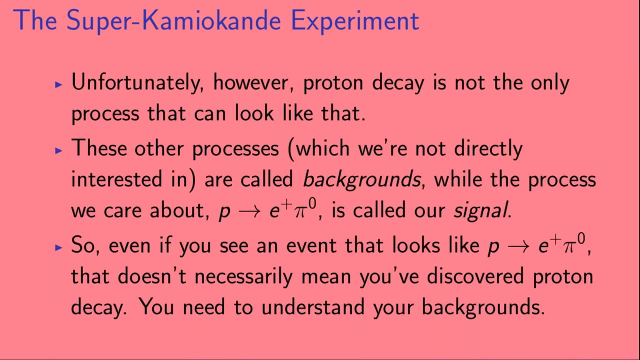 So that's what the decay P goes to. E plus pi-naught would look like in Super-Kamiokande. When something like that occurs, we'll call it an event. Unfortunately, however, proton decay is not the only process that can look like that. 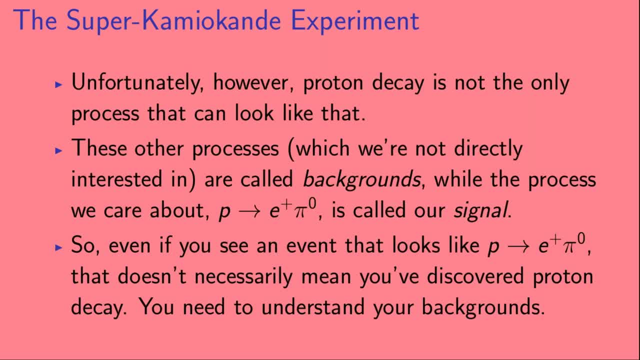 These other processes which we're not directly interested in, are called backgrounds, While the process we care about- P goes to E plus pi-naught- is called our signal. So even if you see an event that looks like P goes to E plus pi-naught, 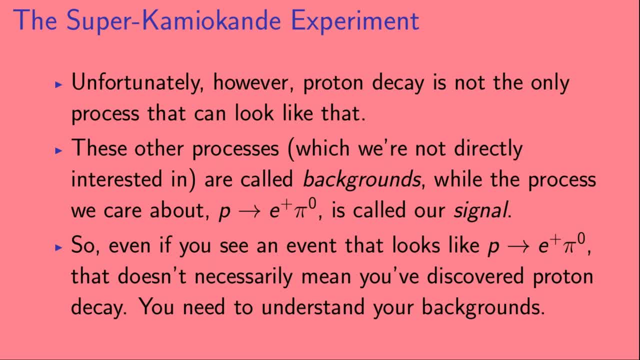 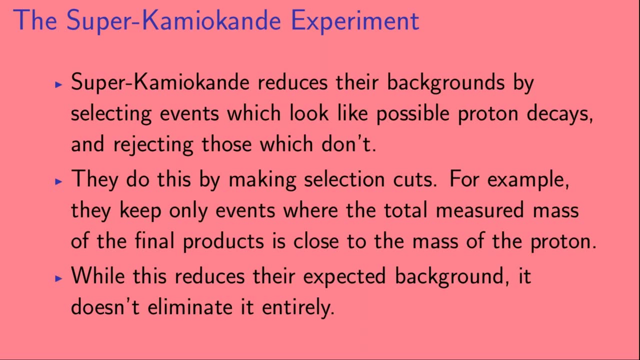 that doesn't necessarily mean you've discovered proton decay. You need to understand your backgrounds. Now Super-Kamiokande reduces their backgrounds by selecting events which look like possible proton decays and rejecting those that don't. They do this by making selection cuts. 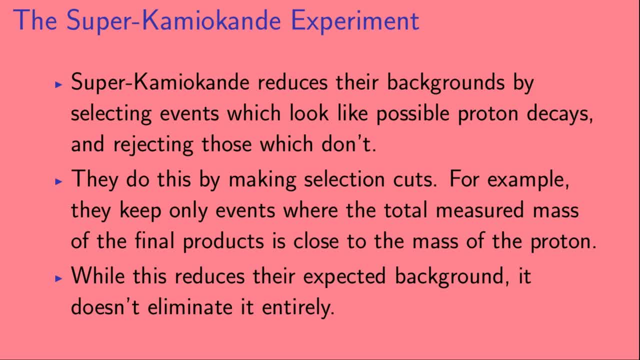 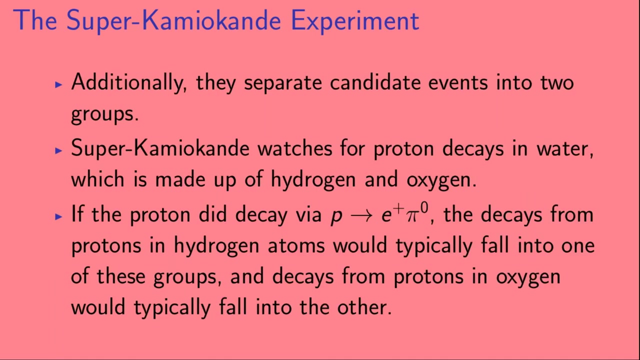 For example, they keep only events where the total measured mass of the final products is close to the mass of the proton. While this reduces their experimental background, it doesn't eliminate it entirely. Additionally, they separate candidate events into two groups. Now Super-Kamiokande watches. 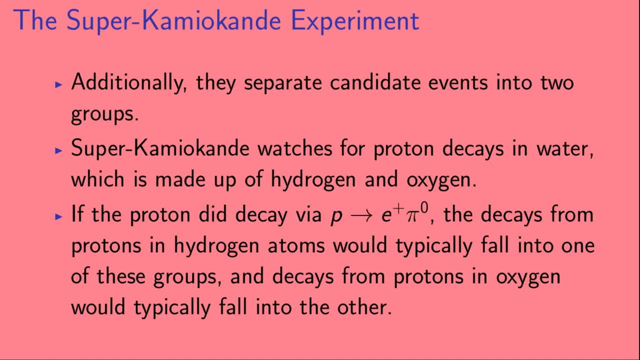 for proton decays in water, which is made up of hydrogen and oxygen. If the proton did decay via, P goes to E plus pi-naught. the decays from protons in hydrogen atoms would typically fall into one of these groups, and decays from protons in oxygen. 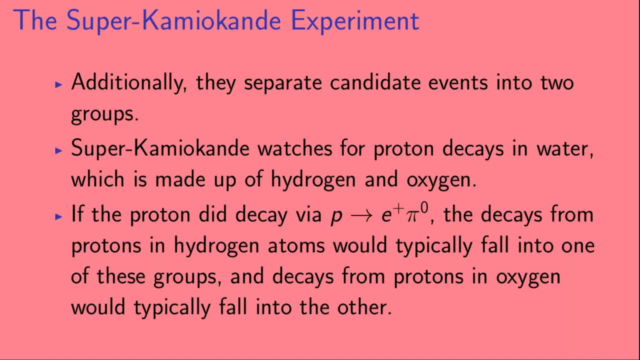 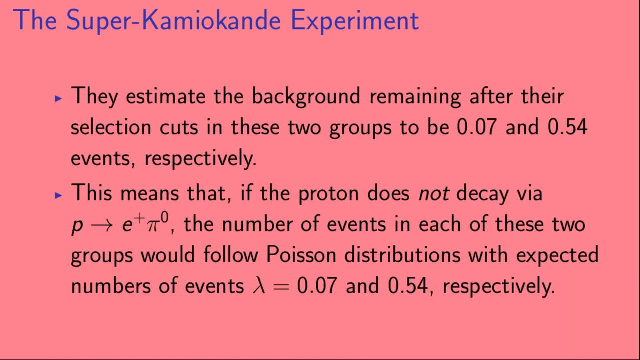 would typically fall into the other. They estimate the background remaining after their selection cuts in these two groups to be 0.07 and 0.54 events respectively. This means that if the proton does not decay via, P goes to E plus pi-naught. 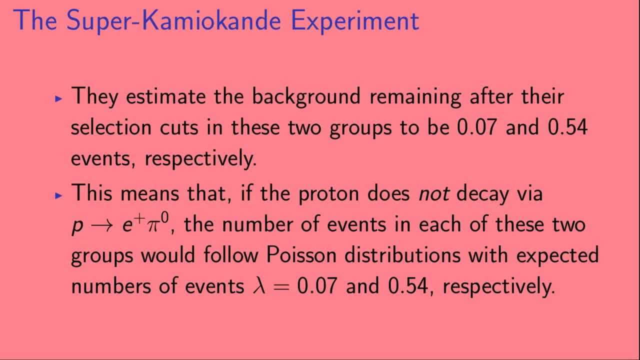 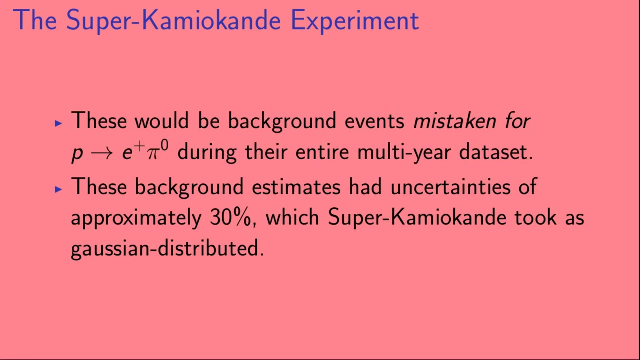 the number of events in each of these two groups would follow Poisson distributions, with expected numbers of events lambda equal to 0.07 and 0.54, respectively. These would be background events mistaken for. P goes to E plus pi-naught during their entire multi-year data set. 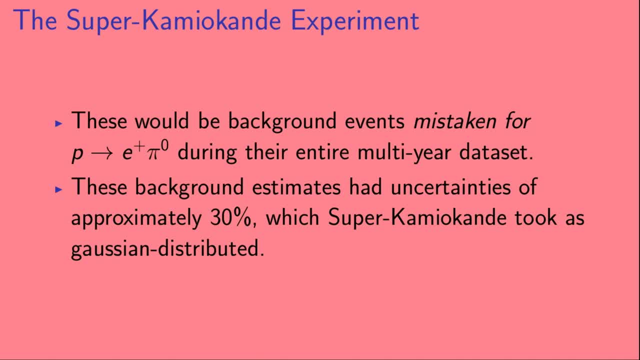 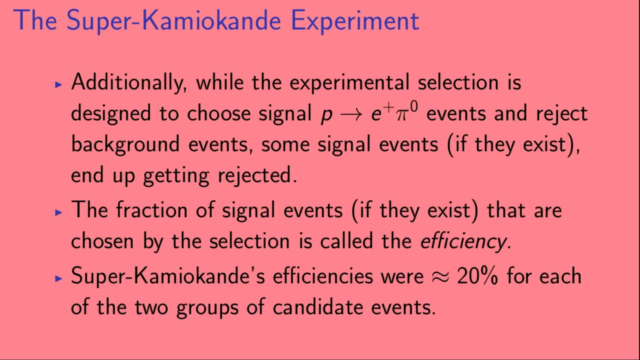 These background estimates had uncertainties of approximately 30% which Super-Kamiokande took as Gaussian distributed. Additionally, while the experimental selection is designed to choose signal P goes to E plus pi-naught events and reject background events, some signal events, if they exist. 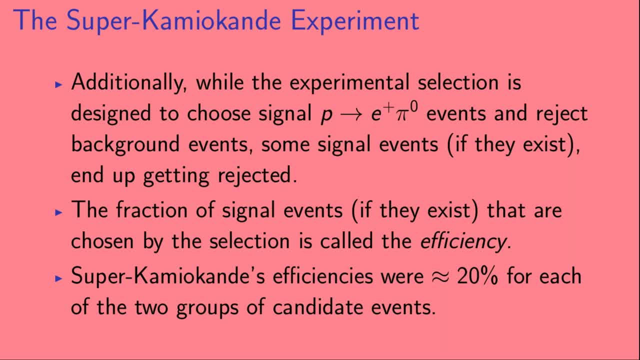 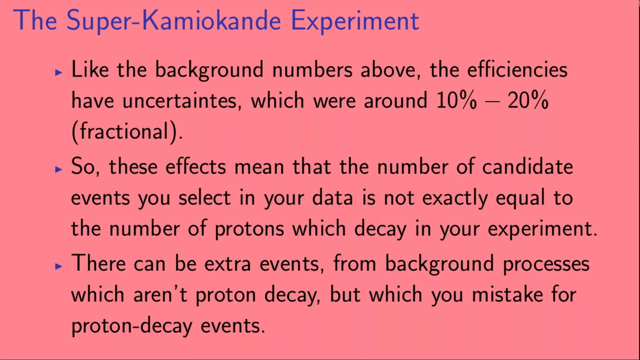 end up getting rejected. The fraction of signal events, if they exist, that are chosen by the selection is called the efficiency. Super-Kamiokande's efficiencies were about 20% for each of the two groups of candidate events. Like the background numbers above, 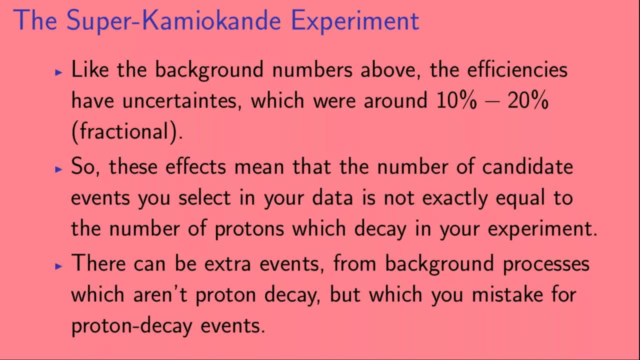 the efficiencies have uncertainties, which were around 10 to 20%. Now, that's 10 to 20% of the efficiencies, which were themselves about 20%. So these effects mean that the number of candidate events you select in your data is not exactly equal to the number of protons. 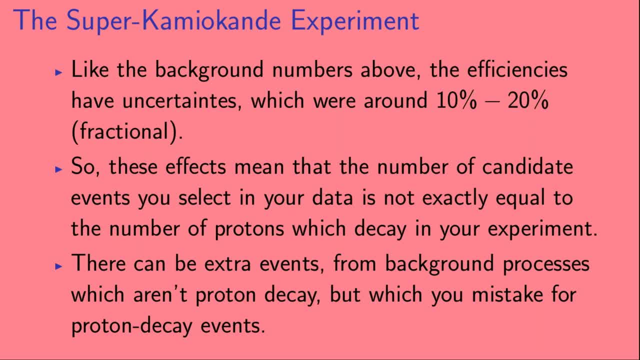 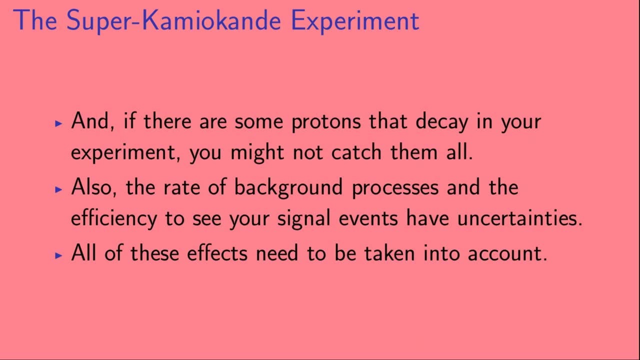 which decay in your experiment. There can be extra events from background processes which aren't proton decay but which you mistake for protons which are not proton decay events. And if there are some protons that decay in your experiment you might not catch them all. 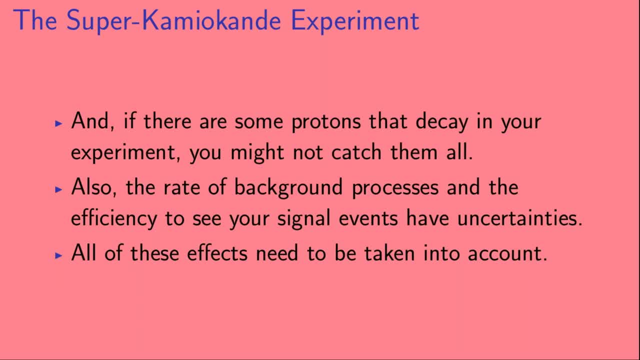 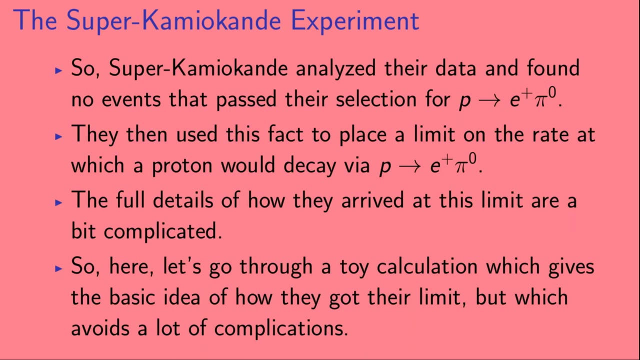 Also the rate of background processes and the efficiency to see your signal. events have uncertainties, So all of these effects need to be taken into account. So Super-Kamiokande analyzed their data and found no events that passed. their selection for p goes to e plus pi-naught. 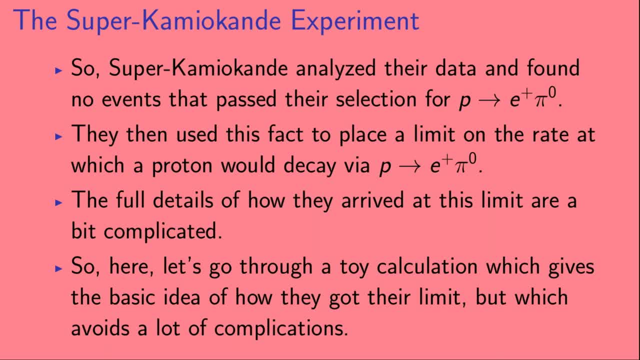 They then used this fact to place a limit on the rate at which a proton would decay via. p goes to e plus pi-naught. The full details of how they arrived at this limit are a bit complicated, So here let's go through a toy calculation. 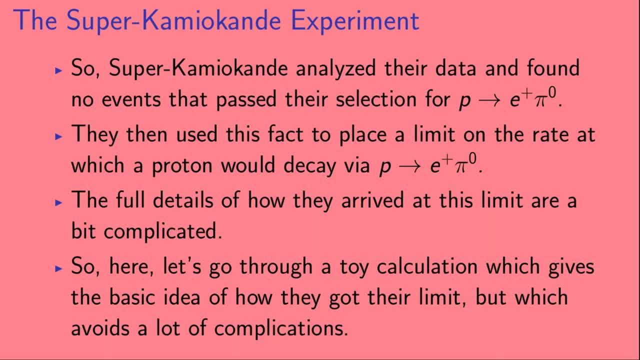 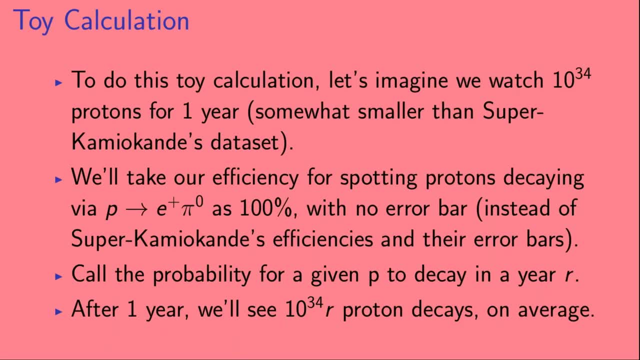 which gives the basic idea of how they got their limit but which avoids a lot of complications. To do this toy calculation, let's imagine we watched 10 to the 34 protons for one year. So this is somewhat smaller than Super-Kamiokande's data set. 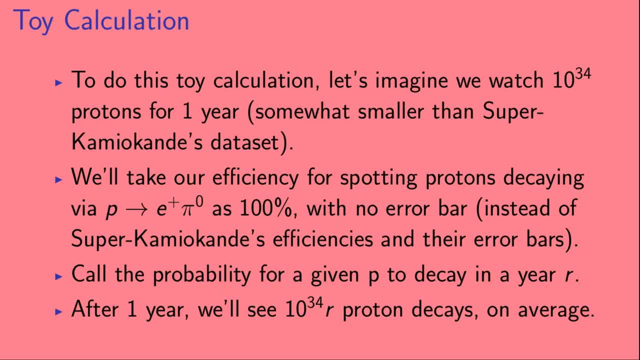 We'll take our efficiency for spotting protons decaying via p goes to e plus pi-naught as 100% With no error bar, Instead of Super-Kamiokande's efficiencies and their error bars. Now let's call the probability for a given proton to decay in a year r. 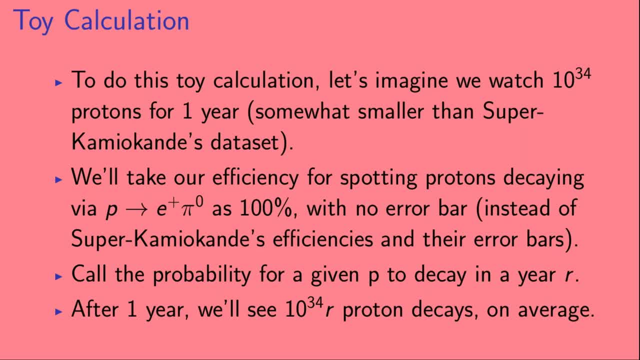 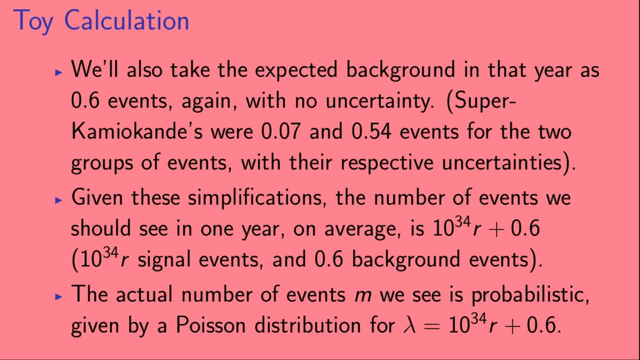 After one year we'll see 10 to the 34 times r proton decays on average. We'll also take the expected background in that year as 0.6 events, Again with no uncertainty. Super-Kamiokande's were 0.07 and 0.54 events. 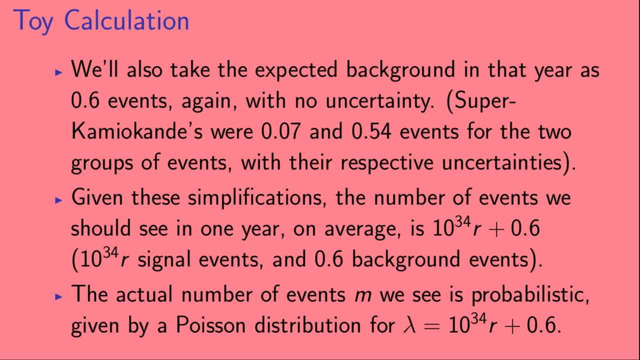 for the two groups of events with their respective uncertainties. Given these simplifications, the number of events we should see in one year on average is 10 to the 34 times r plus 0.6.. So that's 10 to the 34 r signal events. 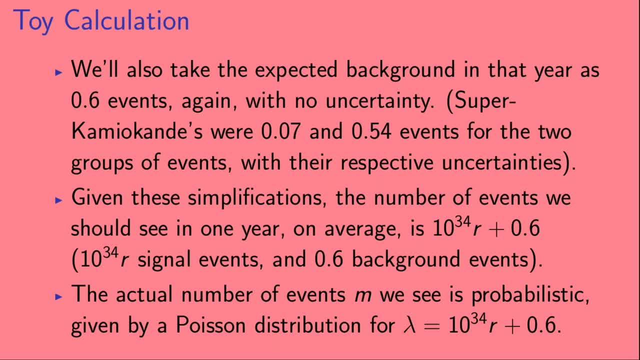 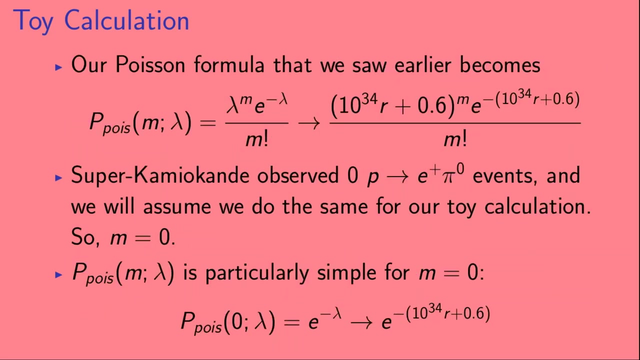 and 0.6 background events. The actual number of events m that we see is probabilistic, given by a Poisson distribution for lambda equal to 10 to the 34 r plus 0.6.. So our Poisson formula that we saw earlier becomes: 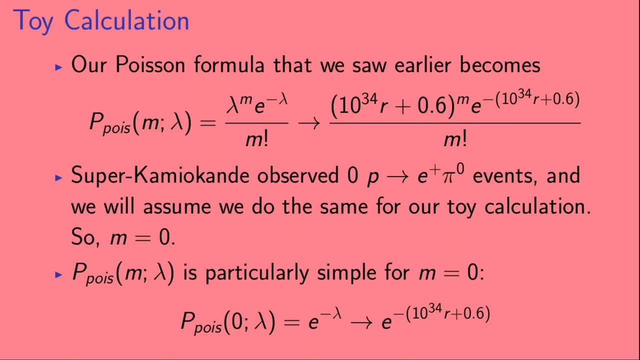 the Poisson probability to observe m events when lambda are expected, which equals lambda to the m e to the minus lambda over m factorial goes to 10 to the 34 r plus 0.6, all raised to the m power e to the minus 10 to the 34 r plus 0.6. 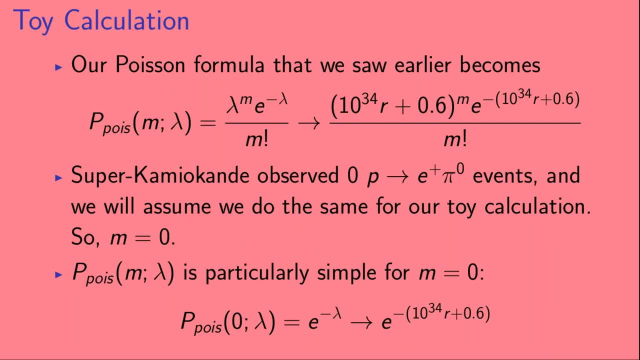 all divided by m, factorial. Now Super-Kamiokande observed, 0 p goes to e plus pi naught events, and we will assume we do the same for our toy calculation. So m equals 0.. Now the Poisson probability: p. Poisson of m, given lambda. 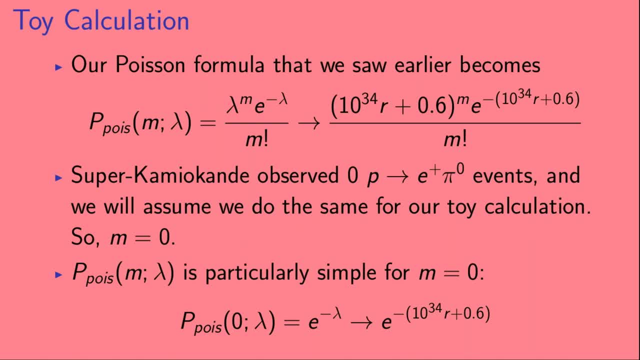 is particularly simple for the case m equals 0.. So the Poisson probability for m equals 0 for some value of lambda equals e to the minus lambda, which in this case is e to the minus 10 to the 34 r plus 0.6.. 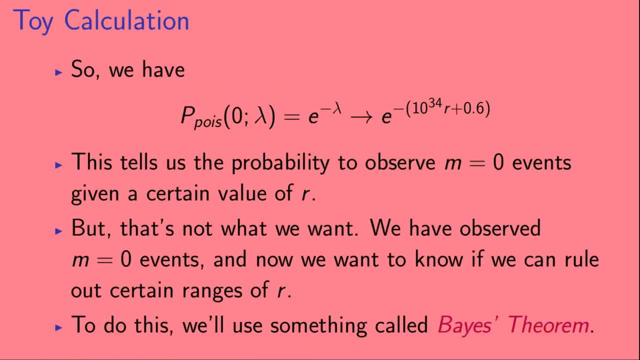 Okay, So we have that our Poisson probability to observe 0 events is equal to e, to the minus 10, to the 34 times r plus 0.6.. This tells us the probability to observe m equals 0 events given a certain value of r. 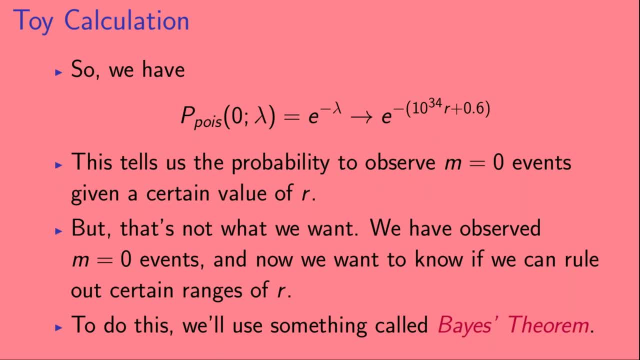 But that's not what we want. We have observed m equals 0 events, and now we want to know if we can rule out certain ranges of r. To do this, we'll use something called Bayes' theorem. Our goal is to make a statement like this. 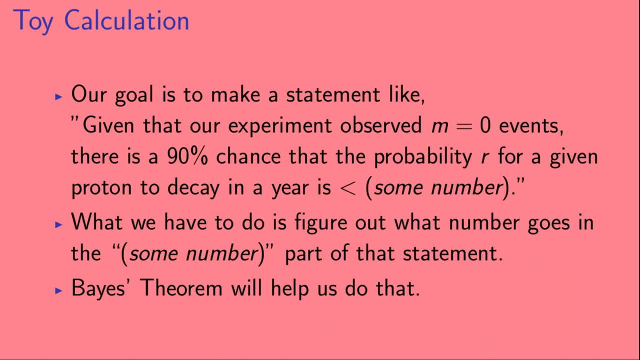 Given that our experiment observed m equals 0 events, there is a 90% chance that the probability r for a given proton to decay in a year is less than some number. What we have to do is figure out what number goes in the some number part of that statement. 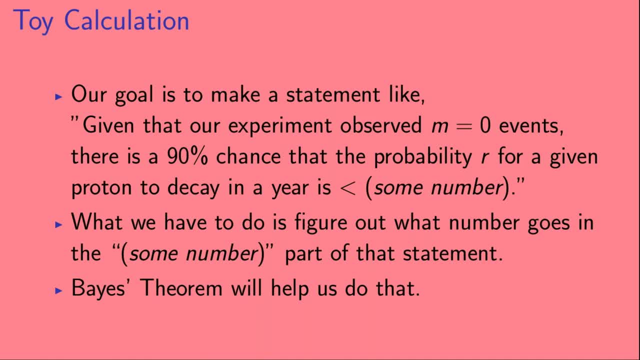 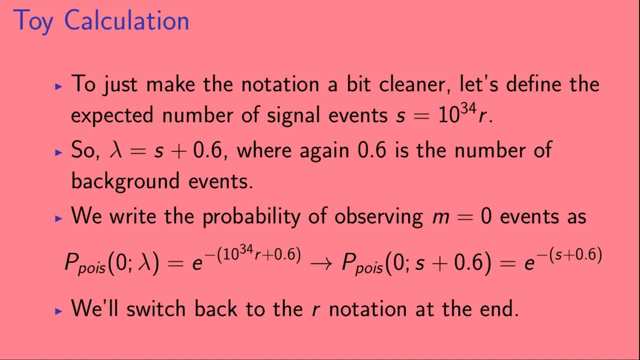 Bayes' theorem will help us do that. To just make the notation a bit cleaner, let's define the expected number of signal events s to be 10 to the 34 r. So lambda is equal to s plus 0.6, where again 0.6. 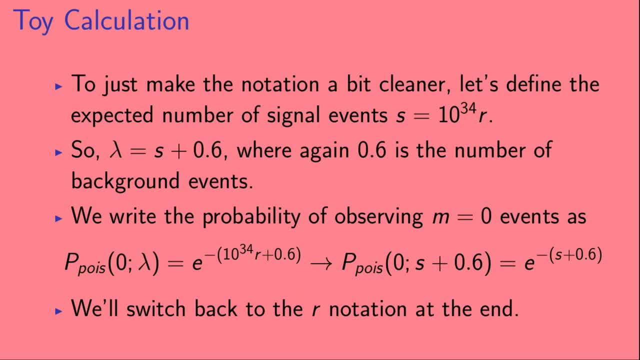 is the number of background events. We write: the probability of observing m equals 0 events as the Poisson probability to observe 0, given lambda, where now lambda is equal to s plus 0.6.. So this is equal to e, to the minus s plus 0.6.. 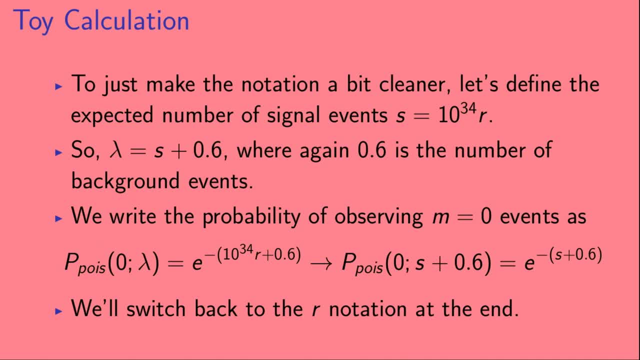 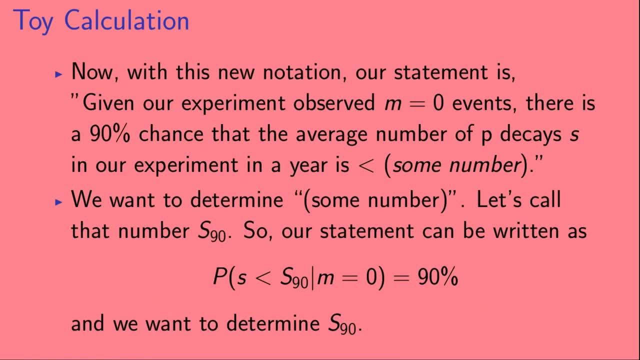 We'll switch back to the r notation at the end. Now, with this new notation, our statement is: given that our experiment observed m equals 0 events, there is a 90% chance that the average number of proton decays s in our experiment in a year. 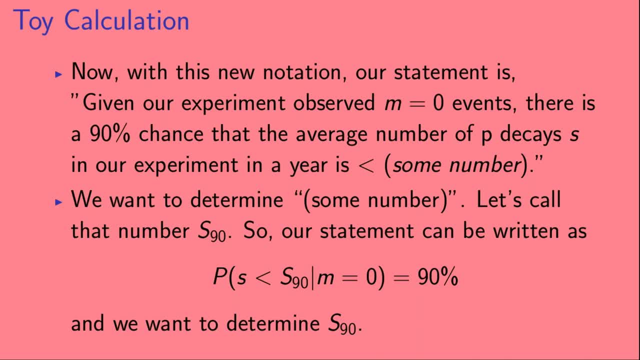 is less than some number. So we want to determine the some number part of that statement. Let's call that number s90.. So our statement can be written as: the probability that s is less than s90, given that m equals 0, is equal to 90%. 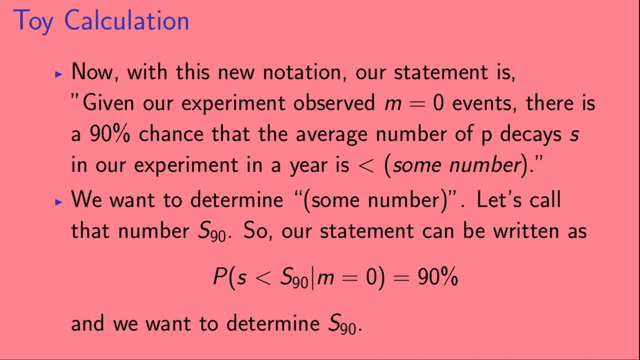 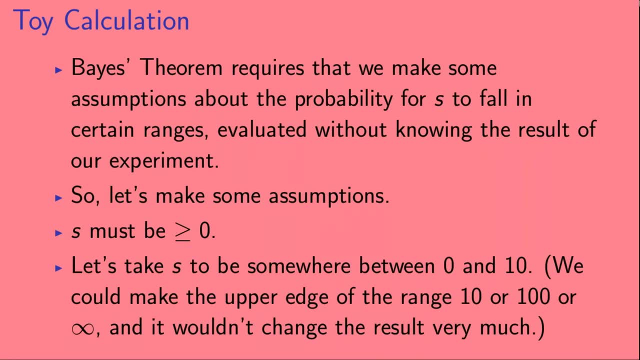 And now our goal is to determine s90.. So Beatty's theorem requires that we make some assumptions about the probability for s to fall in certain ranges evaluated without knowing the result of our experiment. So let's make some assumptions. The number of expected decays. 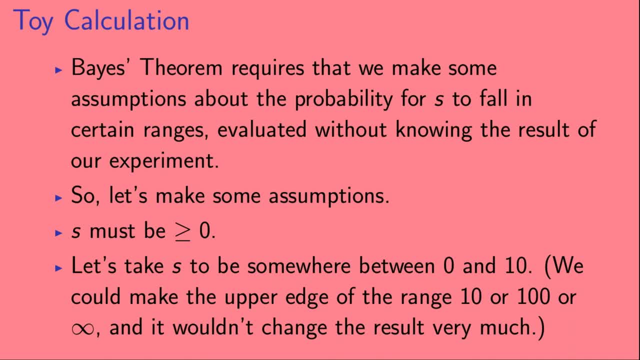 cannot be negative, So s must be greater than or equal to 0.. Let's take s to be somewhere between 0 and 10.. We could make the upper edge of the range 10 or 100 or infinity, and it wouldn't change the result very much. 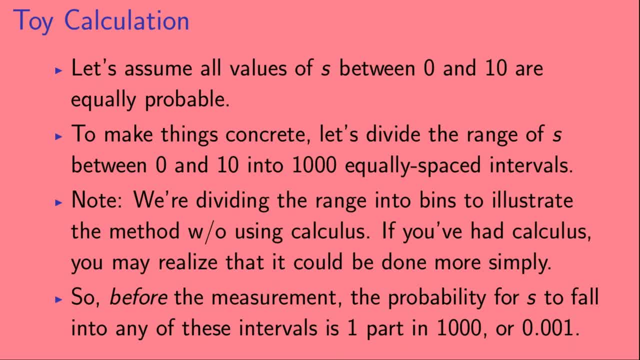 Let's also assume that all values of s between 0 and 10 are equally probable. To make things concrete, let's divide the range of s between 0 and 10 into 1000 equally spaced intervals or bins, And we should note that. 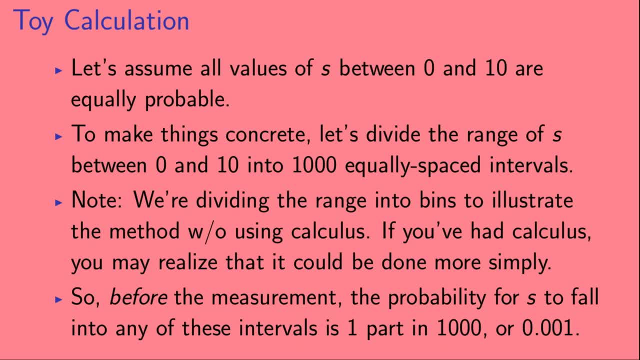 we're dividing the range into bins to illustrate the method without using calculus. If you've had calculus, you may realize that this calculation could be done much more simply. Okay, So before the measurement. the probability for s to fall into any of these intervals is one part in 1000. 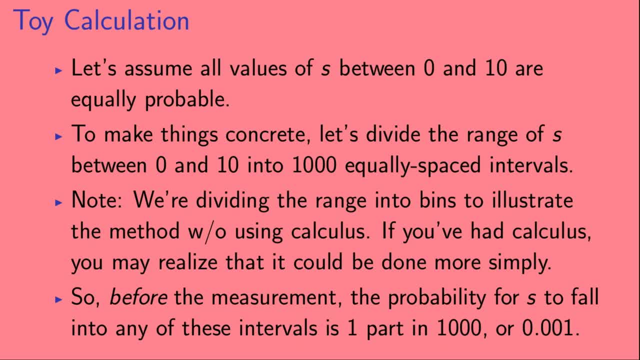 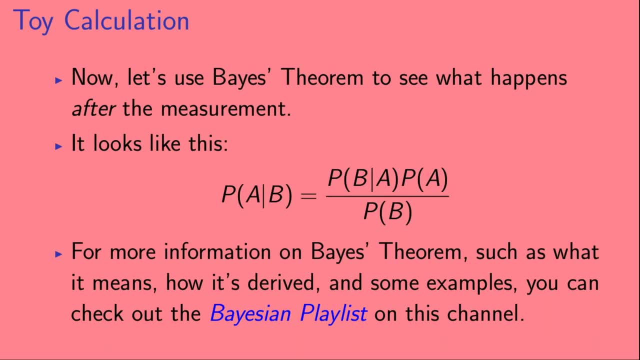 or 0.001.. Now let's use Bayes' theorem to see what happens after the measurement. Bayes' theorem looks like this and it's read as follows: The probability of A given B is equal to the probability of B given A. 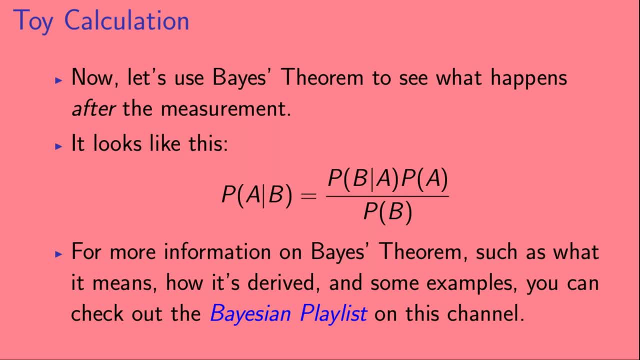 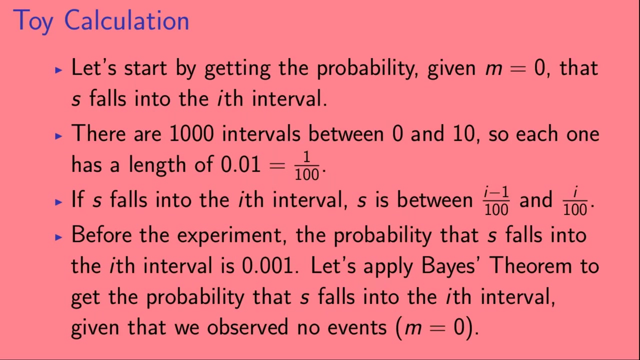 times the probability of A divided by the probability of B. For more information on Bayes' theorem, such as what it means, how it's derived and some examples, you can check out the Bayesian playlist on this channel. Let's start by getting the probability given that. 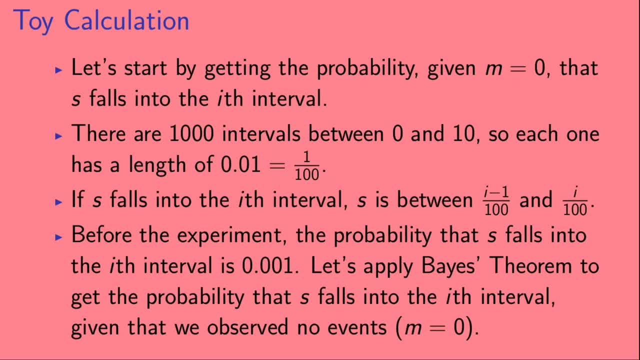 m equals 0, that s falls into the ith interval. There are 1000 intervals between 0 and 10, so each one has a length of 0.01 or 1 over 100.. If s falls into the ith interval, s is between i minus 1 over 100. 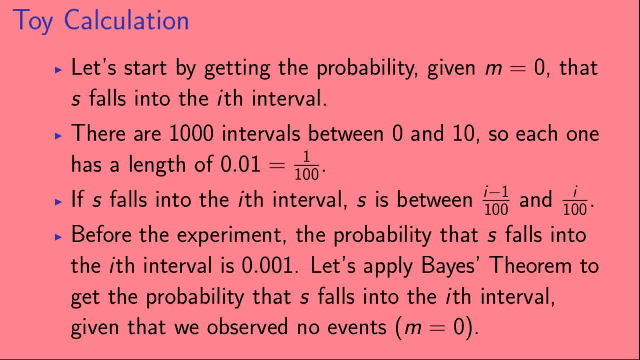 and i over 100.. Before the experiment: the probability that s falls into the ith interval is 0.001, because there are 1000 intervals. Let's apply Bayes' theorem to get the probability that s falls into the ith interval, given that we observed no events. 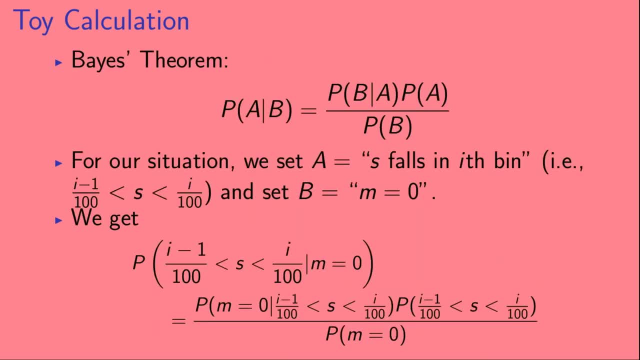 that m equals 0.. Okay, so again, Bayes' theorem says: the probability of A given B is equal to the probability of B given A times the probability of A divided by the probability of B. For our situation we set A equal to s falls into the ith bin. 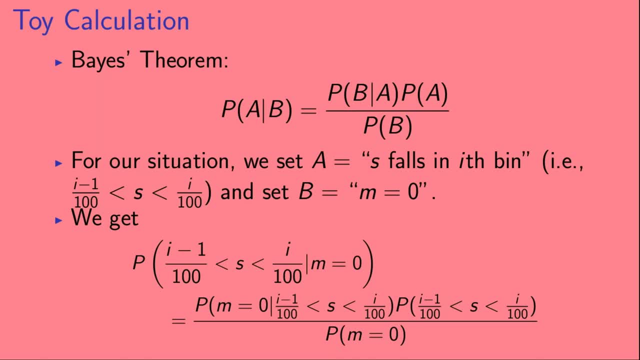 or in other words, s is between i minus 1 over 100 and i over 100. And we set B equal to m equals 0. So we get that the probability that s falls into the ith bin, that's that s is between i minus 1 over 100. 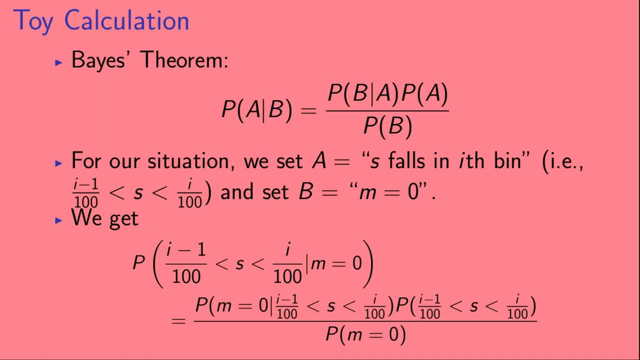 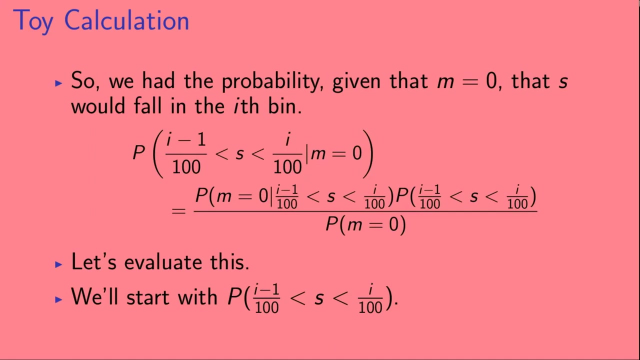 and i over 100. given that m equals 0 is equal to the probability that m equals 0, given that s falls into the ith bin times the probability that s falls into the ith bin, all divided by the probability that m equals 0.. So we had the probability. 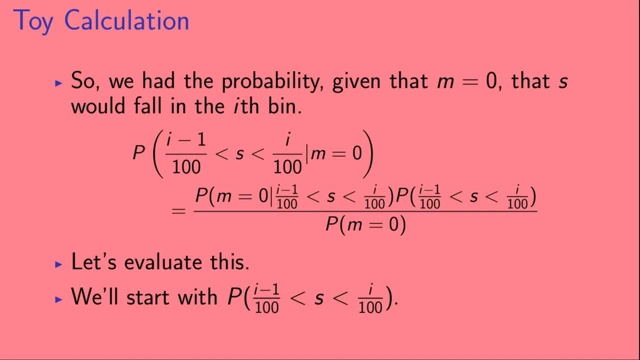 given that m equals 0, that s would fall into the ith bin or, equivalently, that s would be between i minus 1 over 100 and i over 100.. So the probability that s would fall into the ith bin, given that m is equal to 0. 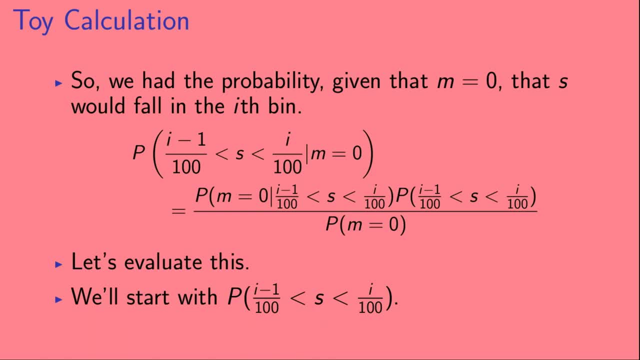 is equal to the probability that m equals 0, given that s falls into the ith bin times the probability that s falls into the ith bin divided by the probability that m would equal 0.. So let's evaluate this. Let's start with evaluating the probability. 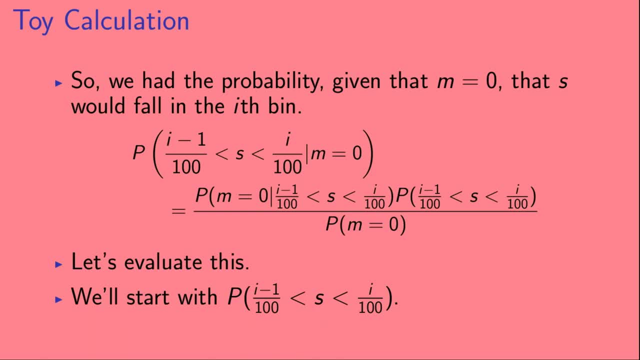 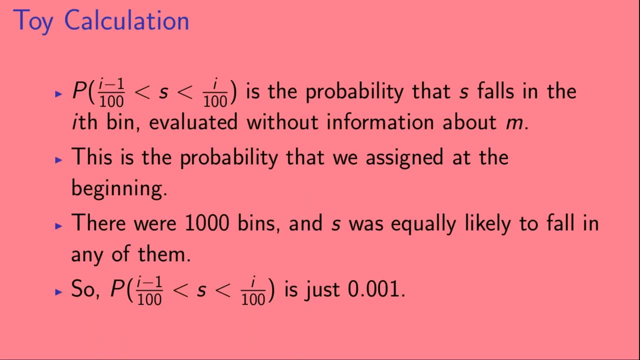 probability that s falls into the ith bin. Now, the probability that s falls into the ith bin is the probability that s falls into the ith bin, evaluated without information about m. This is the probability that we assigned at the beginning. There were 1,000 bins and s was equally likely to fall in any of them. 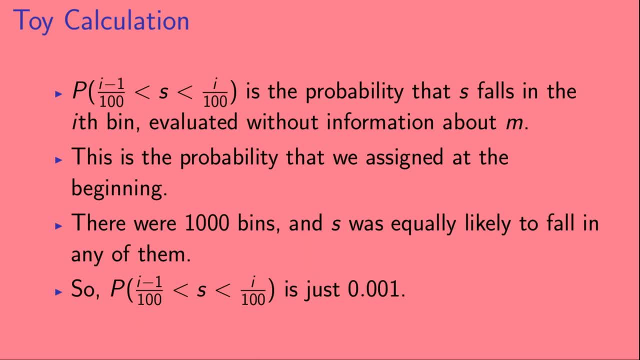 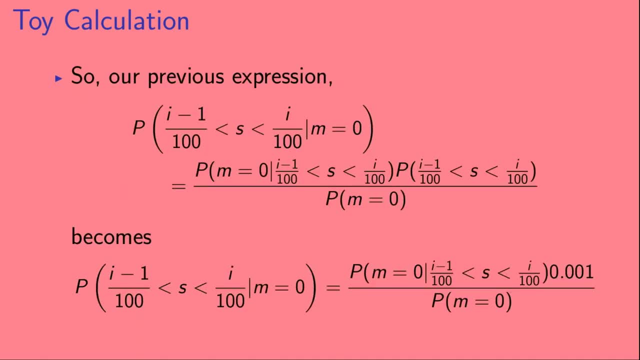 So the probability that s falls in the ith bin is just 0.001, 1 over 1,000.. Okay, so now our previous expression becomes the same thing, except that now we've substituted in for the probability that s falls into the ith bin. 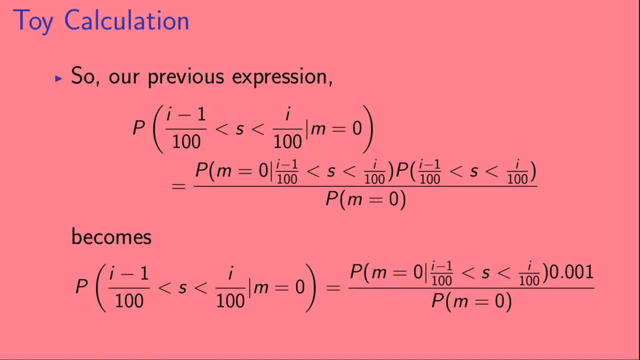 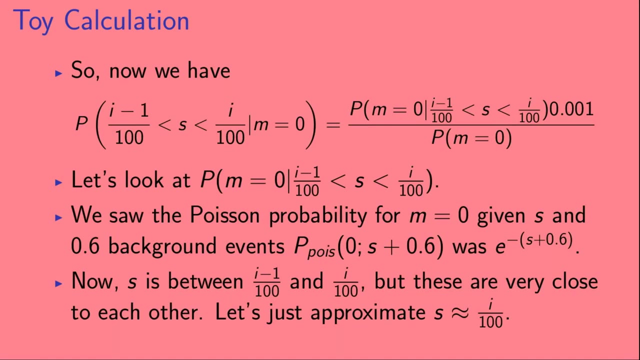 That's the second term in the numerator on the right is now 0.001.. Okay, so now we have that new version of our expression. Let's look at the probability that m equals 0, given that s falls in the ith bin. So this is the first factor in the numerator on the right hand side. 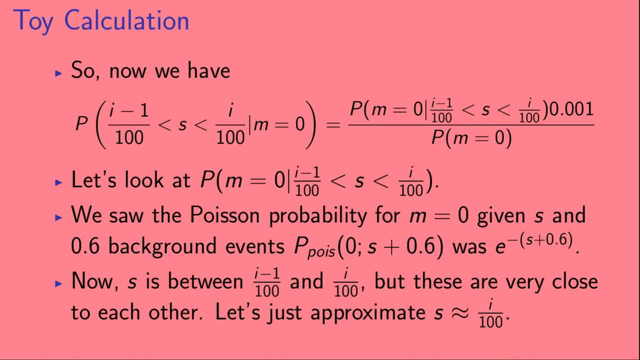 We saw that the Poisson probability to obtain m equals 0, given s and 0.6 background events. the Poisson probability to get 0, given s plus 0.6, was equal to e to the minus s plus 0.6.. 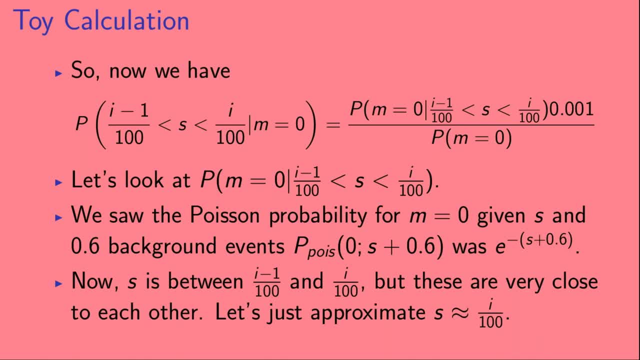 Now here s is between i minus 1 over 100 and i over 100.. But the probability that s falls in the ith bin is 0.001, 1 over 1,000.. Now here s is between i minus 1 over 100 and i over 100.. 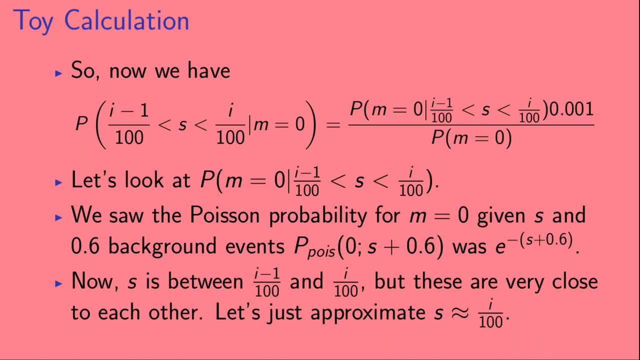 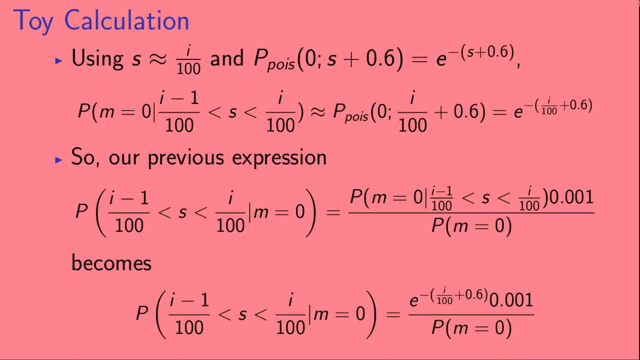 But these are very close to each other. Let's just approximate s as equal to i over 100.. Okay, so using s is approximately equal to i over 100, and that the Poisson probability to observe zero events when s plus 0.6 are expected is equal to e to the minus s plus. 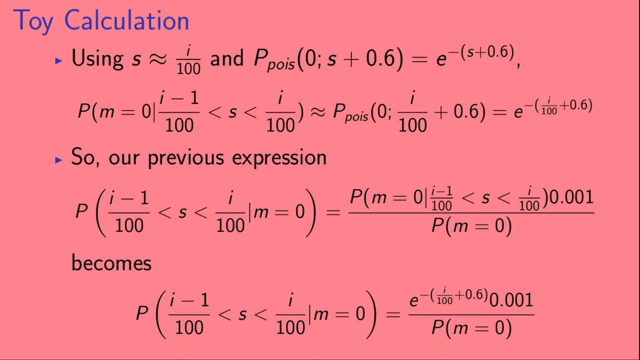 0.6, we get that the probability for m to equal zero, given that s is in the ith bin, is approximately equal to the Poisson probability to observe zero events when i over 100 plus 0.6 are expected, And that equals e to the minus s plus 0.6.. 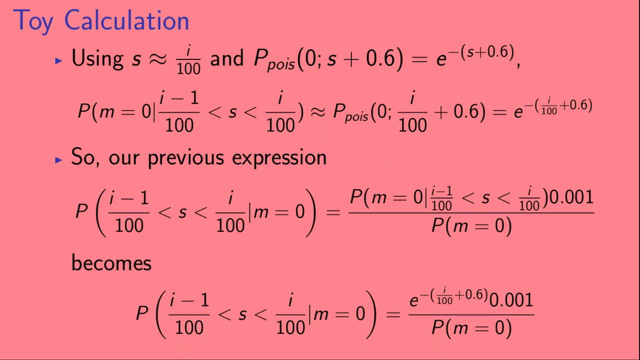 Okay, Okay. So now our previous expression becomes the same thing, except that now on the right-hand side in the numerator we have substituted in e to the minus i over 100 plus 0.6 for the probability that m would equal zero, given that s is in the ith bin. 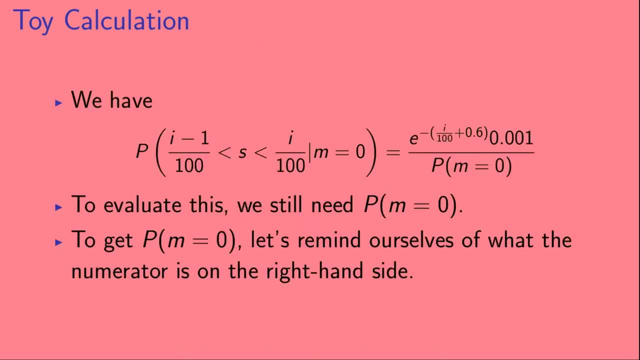 Okay. so now we have the new version of our equation To evaluate this, we still need to get the probability that m equals zero. so the denominator on the right-hand side To get the probability that m equals zero. let's remind ourselves of what the numerator 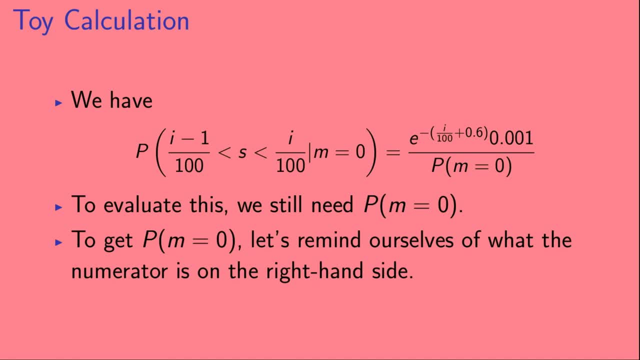 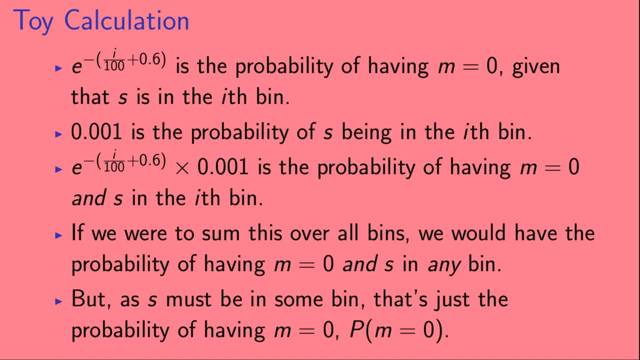 is on the right-hand side. Okay, So e to the minus i over 100 plus 0.6 is the probability of having m equals zero. given that s is in the ith bin, 0.001 is the probability of s being in the ith bin. 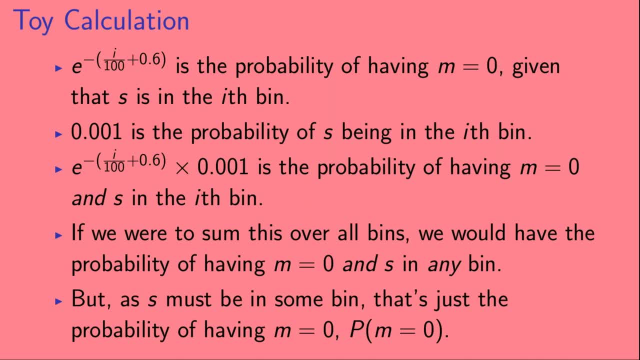 So their product. e to the minus: i over 100 plus 0.6 times 0.001.. E to the minus: i over 100 plus 0.6.. Okay, the probability of having M equals 0 and S in the ith bin. If we were to sum this: 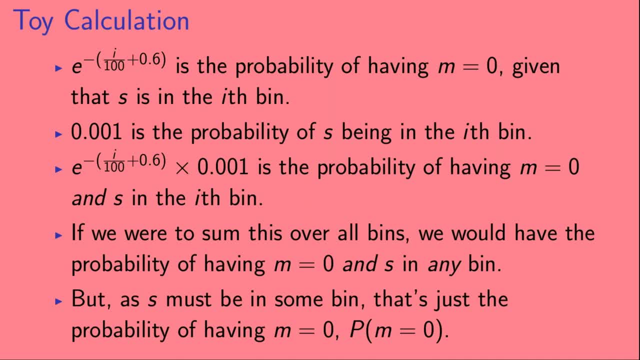 over all bins. we would have the probability of having M equals 0 and S in any bin, But as S must be in some bin, that's just the probability of having M equals 0.. So that's just the probability of M equals 0, which is what we want. 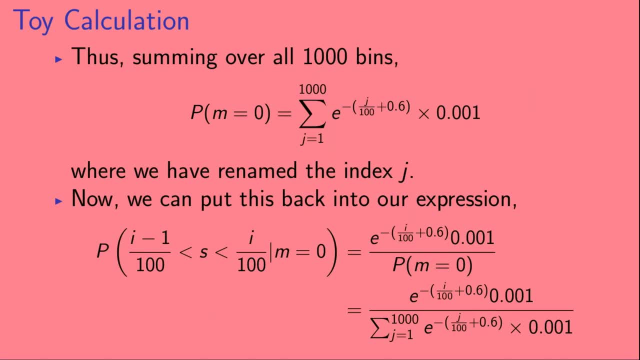 Thus summing over all 1,000 bins, we get that the probability for M to equal 0 is equal to the sum over J from 1 to 100, e to the minus J over 100 plus 0.6 times 0.001, and here: 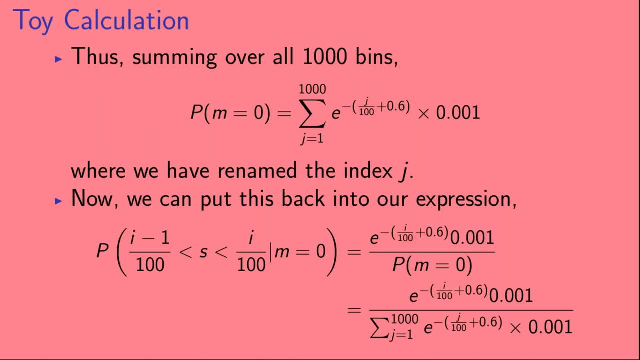 we have renamed the index j, Now we can put this back into our expression. So now we have the probability for s to be in the ith bin. given that m equals 0, is equal to e, to the minus i over 100 plus 0.6 times 0.001, all divided by the. 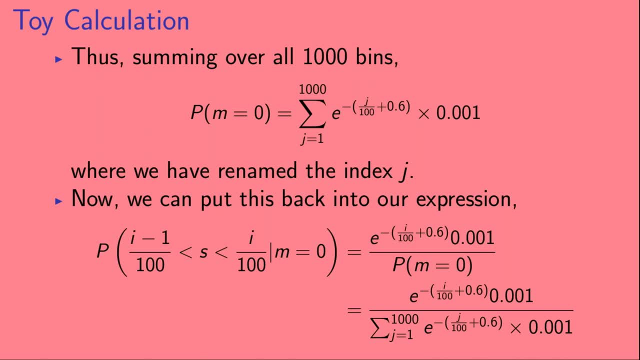 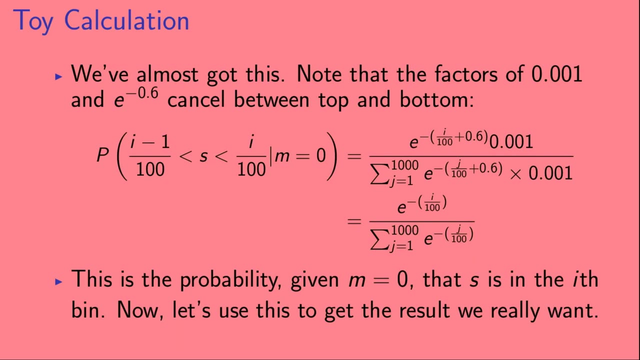 sum over j from 1 to 1,000, e to the minus j over 100, plus 0.6 times 0.001.. Okay so we've almost got this. Note that the factors of 0.001 and e to the minus. 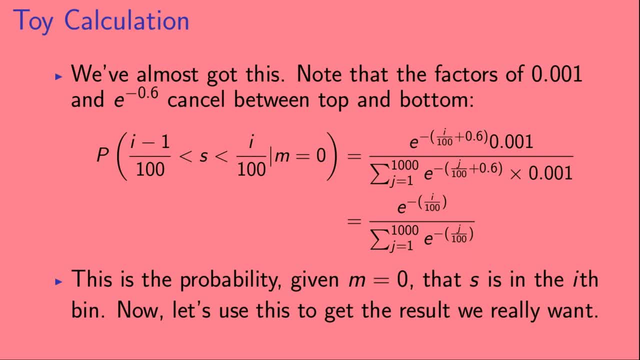 0.6 cancel between the top and bottom. So the probability for s to be in the ith bin is 0.001.. Given that m is equal to 0 is equal to e to the minus i over 100, divided by the sum over j from 1 to 1,000 e to the minus j over 100.. This is the probability. 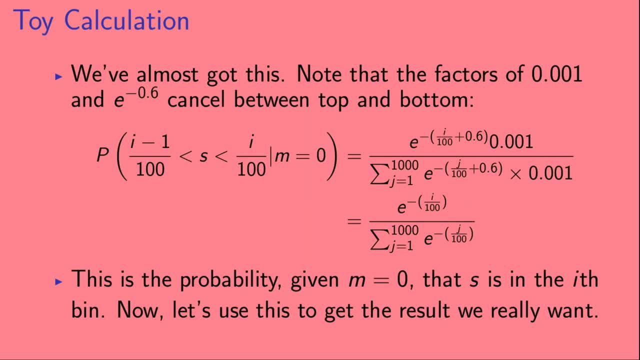 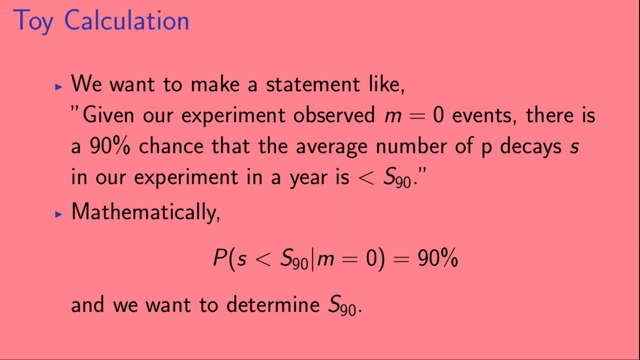 given m equals 0, that s is in the ith bin. Now let's use this to get the result we really want. Okay, so we want to make a statement like: Given that our experiment observed m equals 0 events, there is a 90% chance that the average 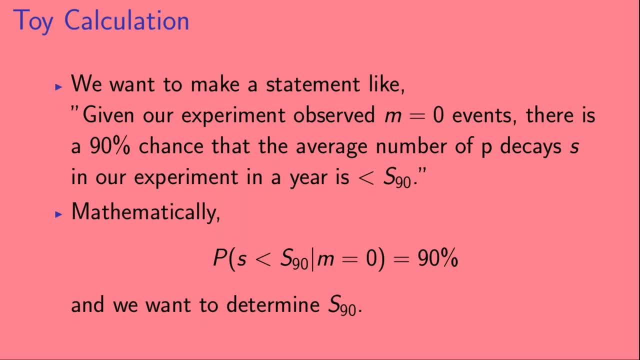 number of proton decays s in our experiment in a year is less than s 90.. Mathematically we say that the probability that s is less than s 90, given the m equals 0, is equal to 90%. Now we need to determine s90. 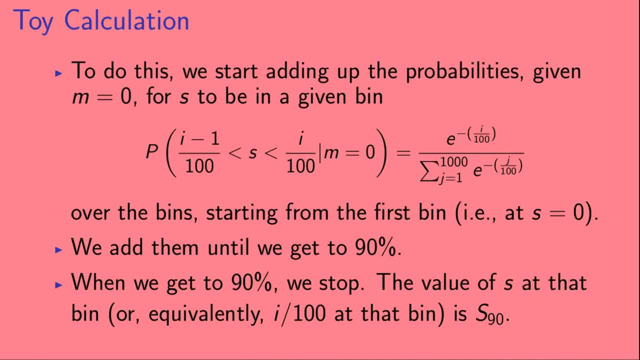 To do this, we start adding up the probabilities- given m equals 0, for s to be in the ith bin over the bins starting from the first bin. so in other words, at s equals 0.. We add up these bins until we get to 90%. 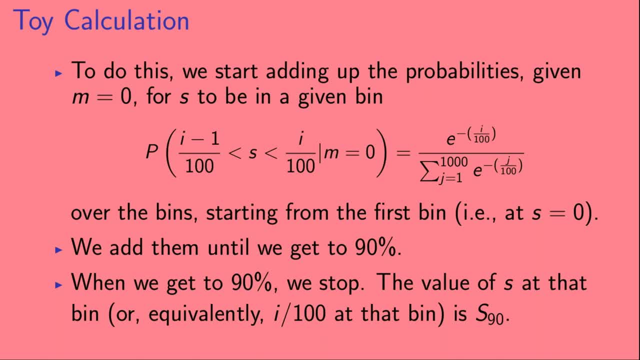 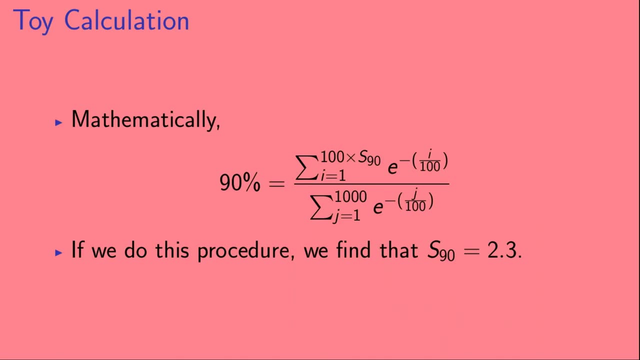 When we get to 90% we stop The value of s at that bin or equivalently i over 100 at that bin is s90.. So mathematically, 90% is equal to the sum over i from 1 to 100 times s90, e to the minus. 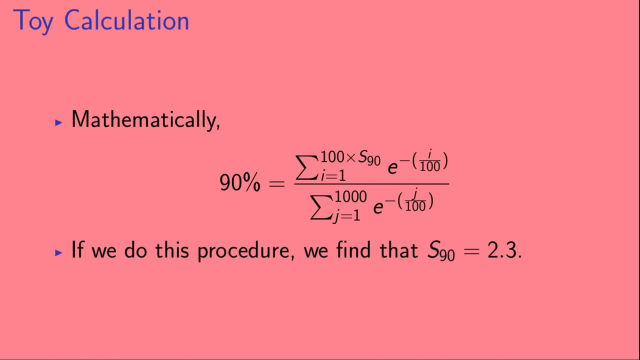 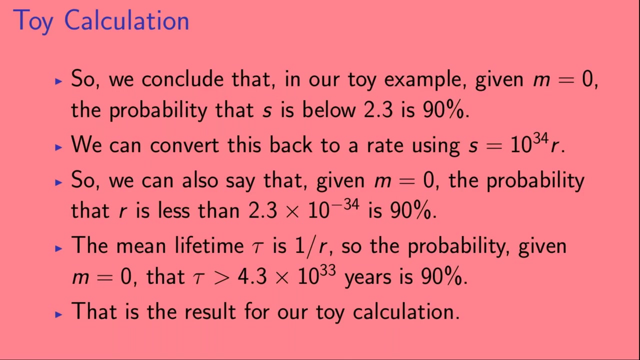 i over 100.. Divided by the sum over all bins j e to the minus j over 100.. If we do this procedure, we find that s90 is equal to 2.3.. So we conclude that in our toy example, given m equals 0, the probability that s is below. 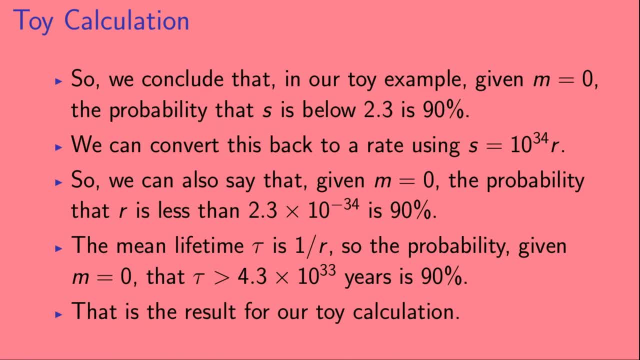 2.3 is 90%, So we can also say that given m equals 0,, the probability that r is less than 2.3 times 10 to the minus 34 is 90%. The mean lifetime tau is 1 over r, so the probability given m equals 0, that tau is. 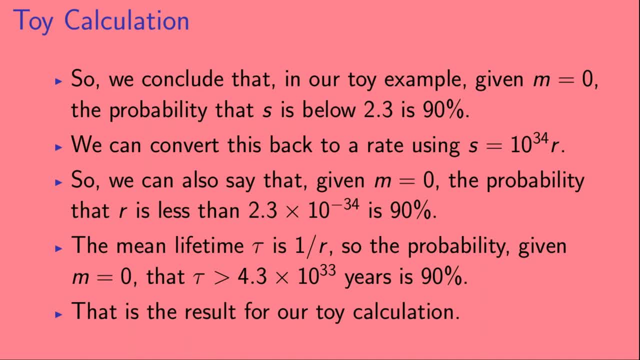 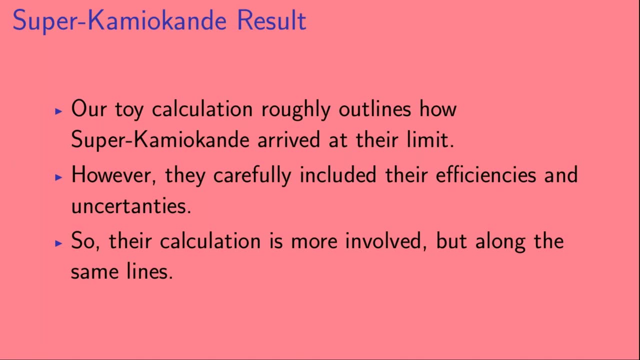 greater than 4.3 times 10 to the minus 33 years is 90%. That is the result for our toy calculation. Our toy calculation roughly outlines how Super-Kamiokande arrived at their limit. However, they carefully included their efficiencies and uncertainties. 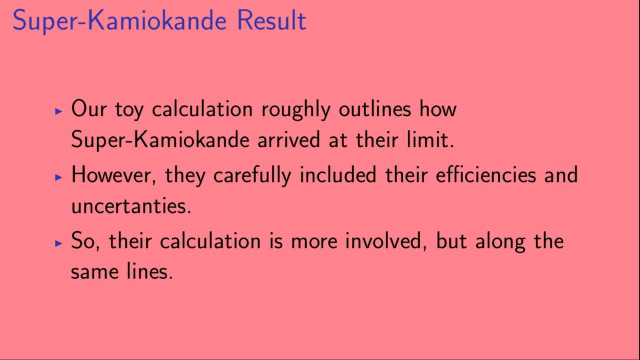 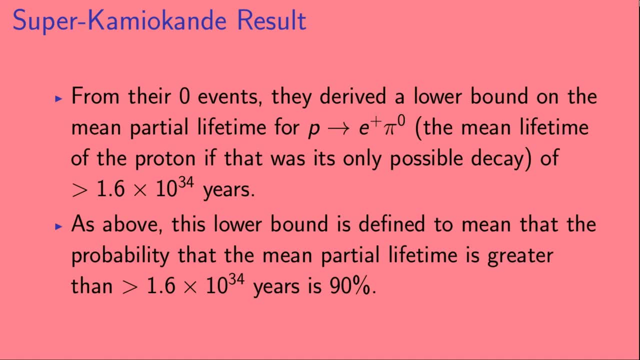 So their calculation is more involved. but along the same lines From their zero events They derived a lower bound on. the mean partial lifetime, for p goes to e plus pi-naught, so that's the mean lifetime of the proton, if that was its only possible decay, of 1.6 times.